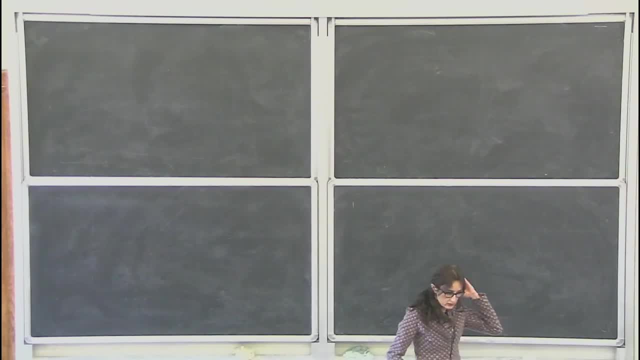 Okay, so this is our last lecture together, and my plan is twofold- is to finish the topic that I started yesterday and that you also developed during the exercises given by Francesca, which is related to gamma rays, And then we will come back a little bit on the transport equation, find the way to solve it and see some results from experiments and from groups that try to interpret the most recent data, if we have time to do everything, 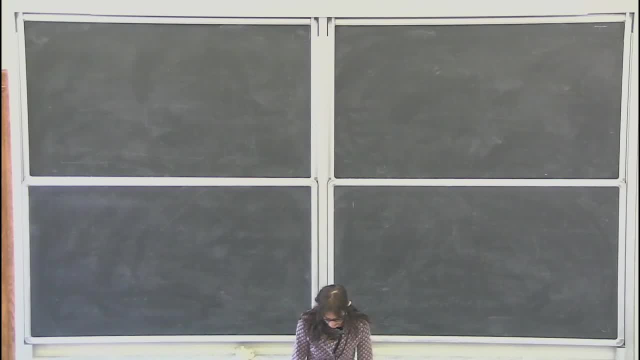 So, going back to gamma rays, I would like to discuss. I would like to discuss the gamma ray sky as we know today. Today it means 2018, 2019.. So the gamma ray sky is being measured in the best way that we have so far by an experiment which has been sent to space by a rocket in 2008.. 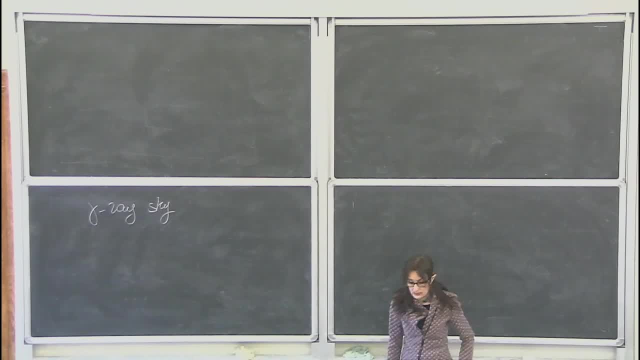 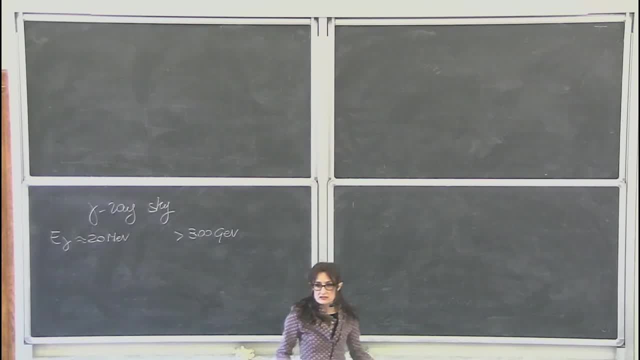 In this energy range the photons arrive at the detector with, of course, I mean. what I wanted to say is the contrary. The detector has an angular aperture, an angular resolution, which changes with energy. So the photons that arrive on the Large Area Telescope are not all once detected with the same precision. 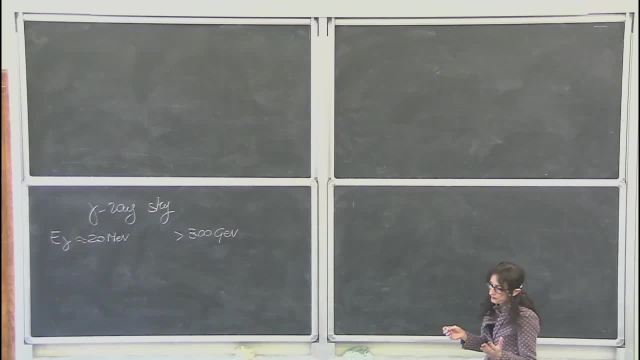 So the photons that arrive on the Large Area Telescope are not all once detected with the same precision. So the photons that arrive on the Large Area Telescope are not all once detected with the same precision. So for purposes linked to dark matter searches and the understanding of sources in the sky, 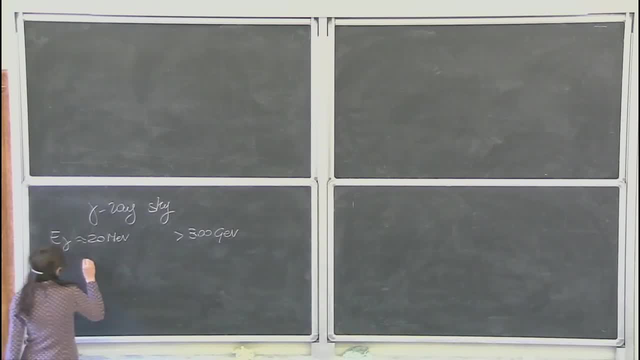 usually one considers energy above 100 MeV. Nevertheless, I don't want to tell you any technical details of this experiment. It is not just the place. Just know that It takes data in an all-sky mode, So every one hour and a half it completes an orbit. 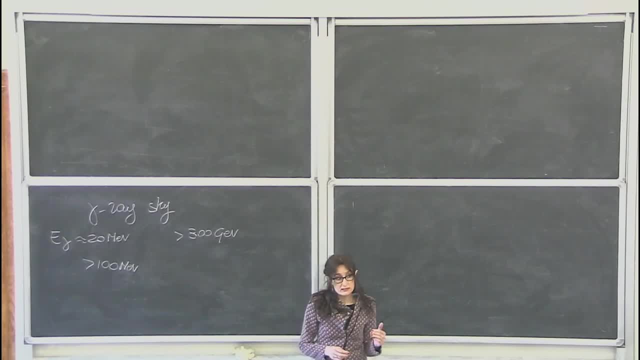 And it has a 70 degrees half angle of view, So any point of the sky is seen by Fermi for half an hour every two orbits, So every three hours. So it is really a great opportunity For me. the first part is a famous Mendelian. 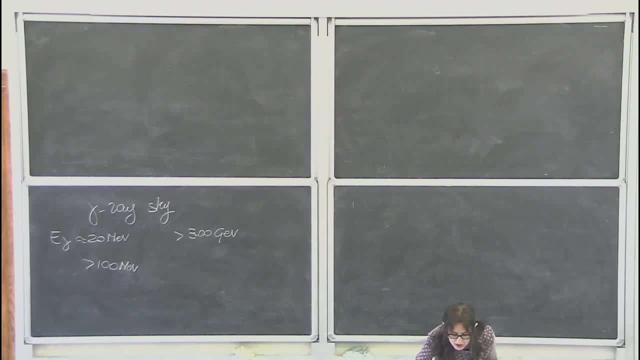 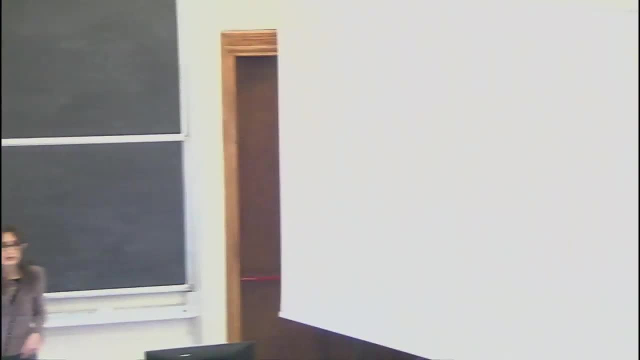 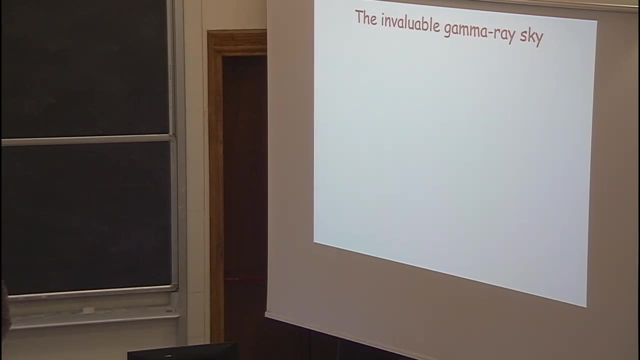 Is that practice Or what's that application? But this particular example is also interesting. It is a very light and mechanical analysis And very Peace-like, led by the use of the히 astroparticle zucches At some point in history機igkeiten стали орεқρονиш었는데. 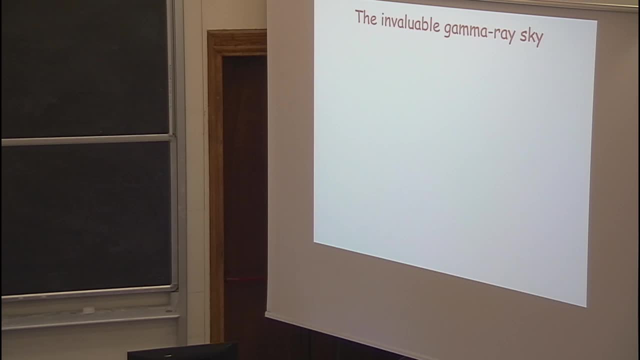 that astro-particle physicists have since the Fermilab antennű analyze Fermi-like data in principle can be. The collaboration puts a lot of software for elaborating the data. so also myself and my collaborators who are not- or at least not all- in the Fermi collaboration. 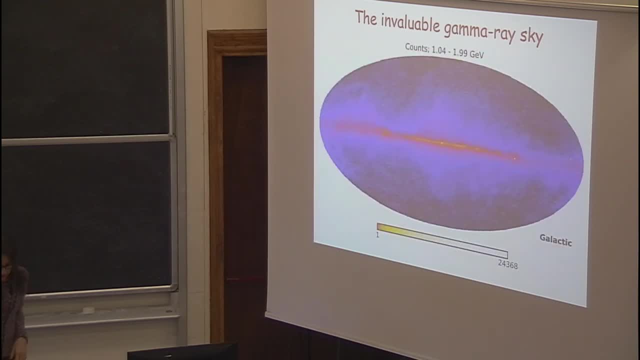 can do this kind of analysis. So this is the all-sky view seen by Fermi between one and two GV. This is the number of photons in each pixel. So here the counts are much, much higher. and this is the galactic disk with all the gas. 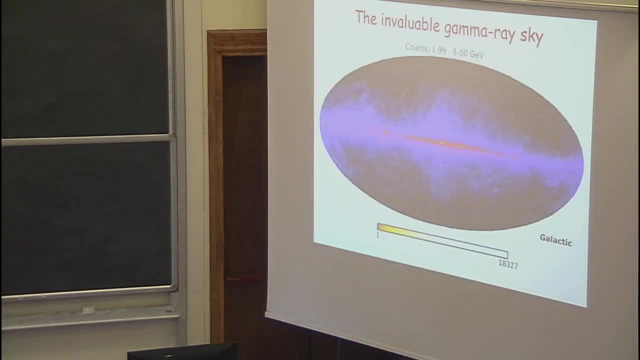 and all the sources. And this is the same sky, but another energy beam, between two and five GV. And this is the sky. well, maybe it's not so clear, but it is much, much darker between five and 10 GV. 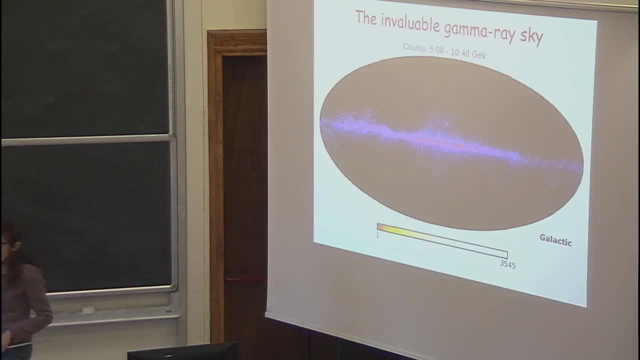 so increasing the energy. Fermilat receives less photons And this is due to the physics of the sources. Normally, the sources of gamma rays, cosmic rays as well, have energy-dependent source spectra that go as a power law. So this is the physics that explains why the physics 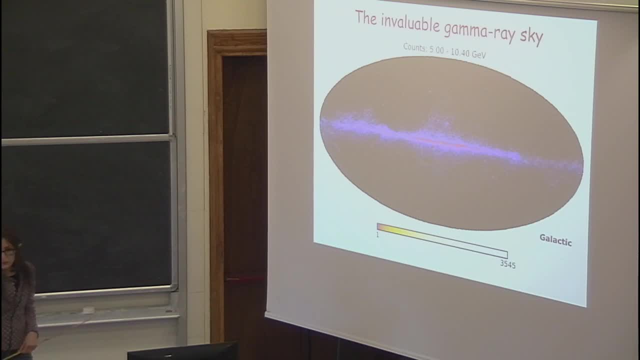 some hint, of course. that explains why this figure is getting darker and darker, And with increasing energy. So the photons now are at most 3,000, so 1,500 per pixel, And at higher energies, you see they were a significant factor higher. 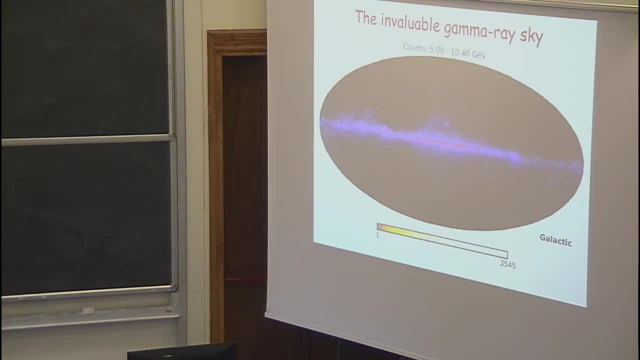 So let me discuss how these photons are produced in the sky. So these are all sky-high, These are sky-high photons coming from any source, any possible dark matter, annihilation and whatever. So let's see together the gamma ray emission And this is you will see in a while. 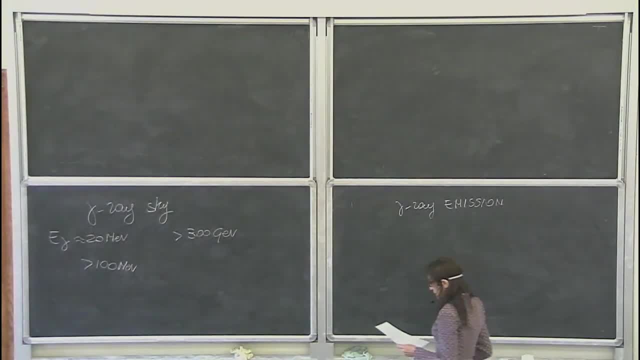 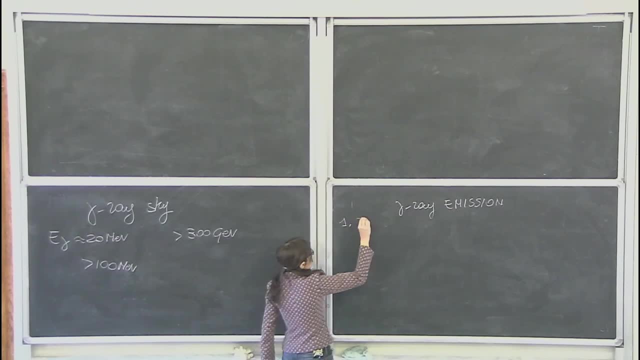 strongly linked to what we have seen in the previous lectures. So the gamma ray emission is predicted. it is a very important factor for the interactions of cosmic rays with galactic gas, And this galactic gas is atomic hydrogen ionized with their isotropic concentration. 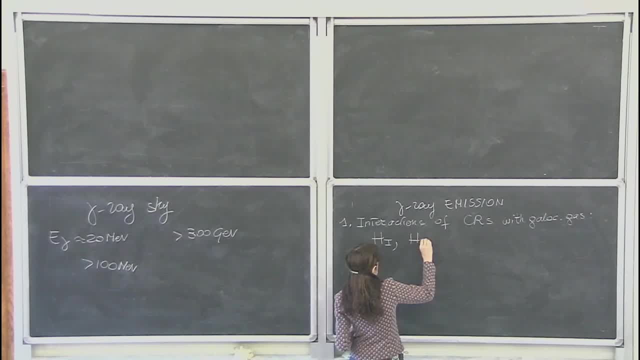 And this is because the gas that is in the ocean- the cosmic race, if you will- is a cosmic gas. So it's a cosmic gas- ionized hydrogen and some gas which escapes most of the observation, which is called dark neutral gas. 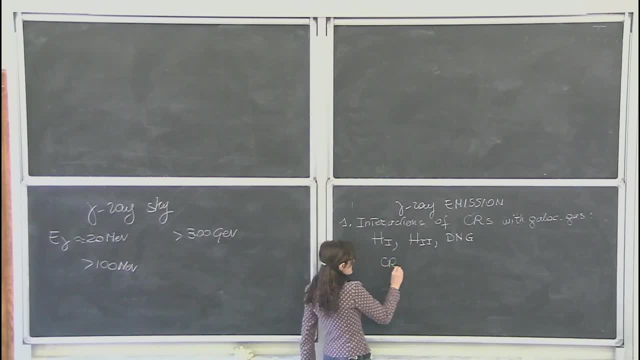 And the interaction is that a cosmic ray, and mostly proton and helium in the cosmic radiation plus one molecule of gas or one proton, undergoes a totally inelastic interaction and hadronic processes occur that then give rise to pi zero plus anything. 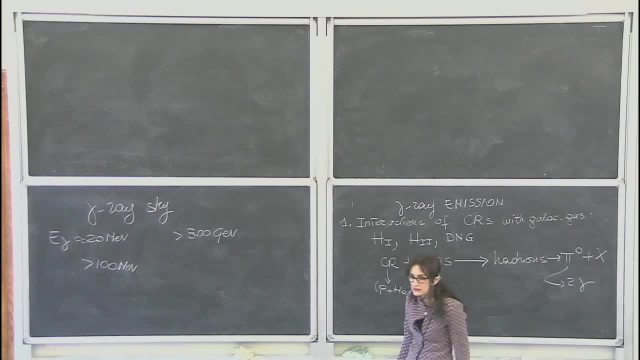 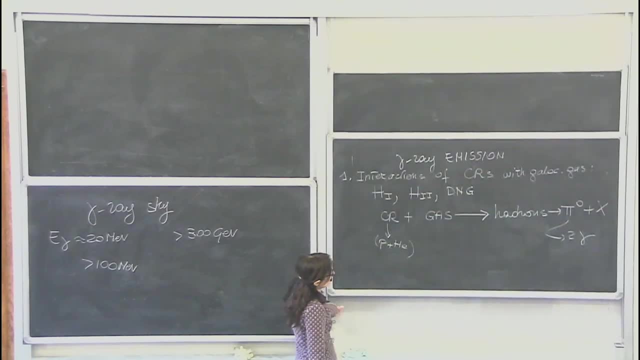 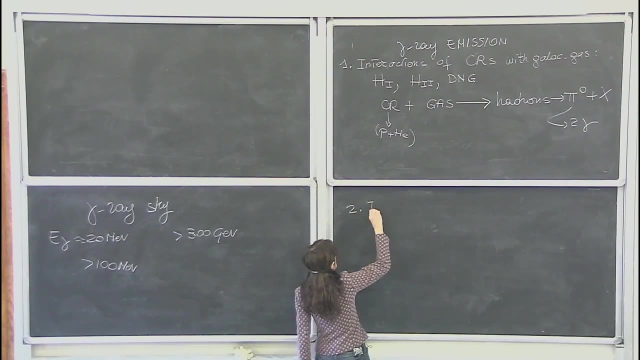 and this pi zero immediately decays into photons And then we have in the sky the inverse Compton emission We have seen a few days ago. So if electrons lose energy by inverse Compton, on the other side we have photons in the gamma-ray sky. 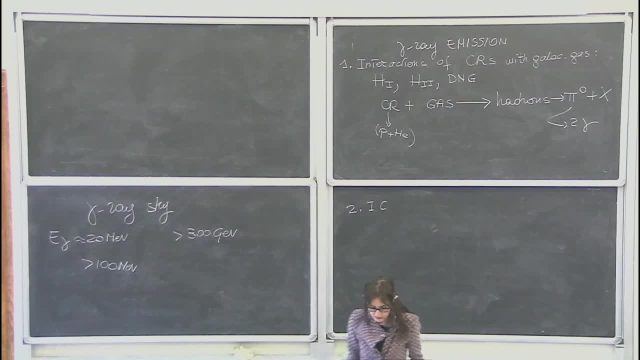 that have been upscattered in energy by these electrons, And so for cosmic rays, so electrons in cosmic rays that interact with the interstellar radiation field. So I remind you that an electron plus a photon with some energy is interacting at the electron up-scatters the photon. 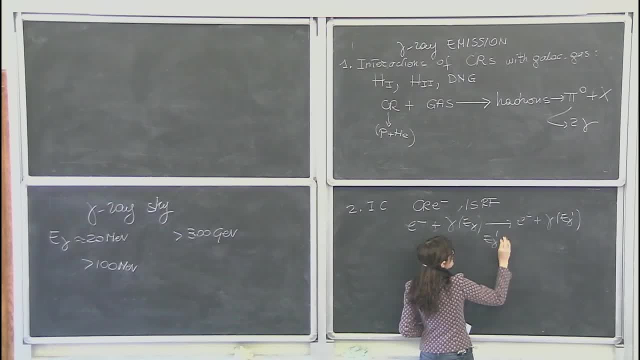 So the energy of the final state photon is greater than the starting energy. Good, Then we have an emission which is measured to be isotropic, And it is particularly visible when studying the gamma-ray sky at high latitudes, And this isotropic emission is very likely. 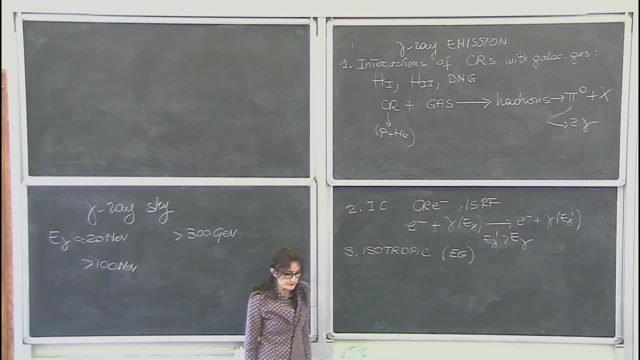 of extragalactic emission origin And it is again a background or it depends what we want to say, we want to study, but it is present everywhere because, since it is very likely of extragalactic origin, every point you move your telescope it is there. 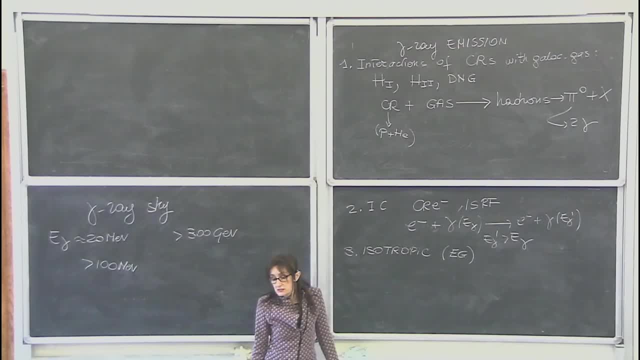 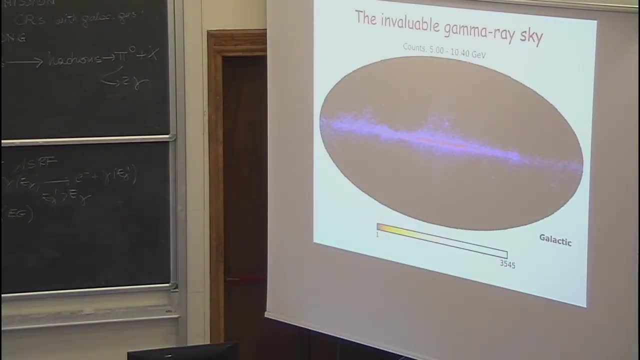 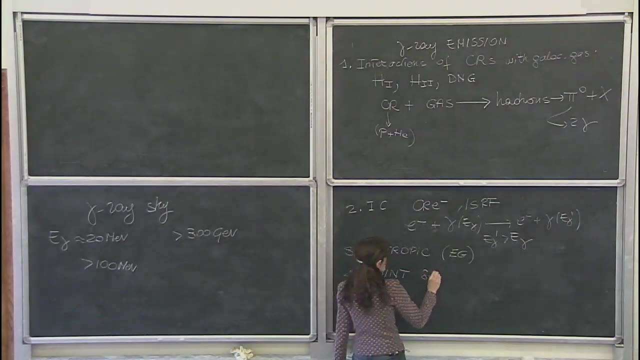 All these emissions that I brought the blackboard are diffuse emissions, so there is not a specific point source, But we know that the telescope has measured a very large number of point sources And, a few days ago, the Fermilab collaboration. 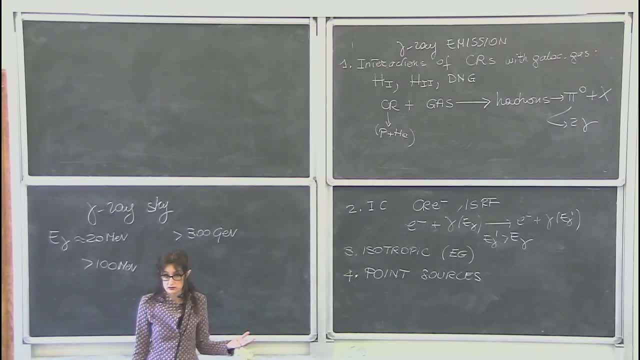 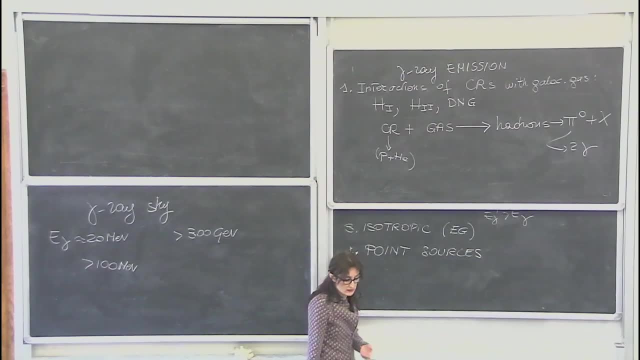 has published the fourth source catalog. You can find the paper on archive And in this release they have analyzed eight years of data. It is not that trivial to analyze, It is data. so they have this result on the first eight over ten years of data. 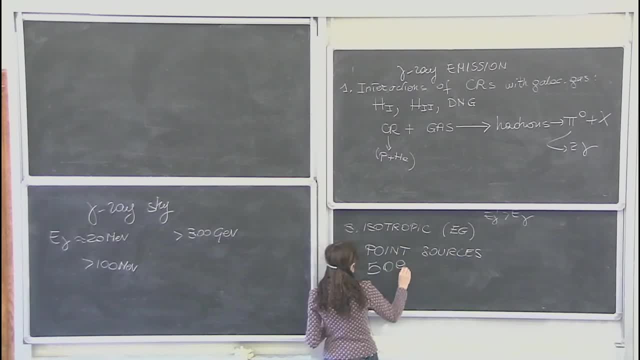 And they have measured 5,098 sources, which is of course the biggest gamma-ray catalog that we have so far. Among these sources there are 17,- sorry, 75 sources which are even extended, So they are not measured as point sources. 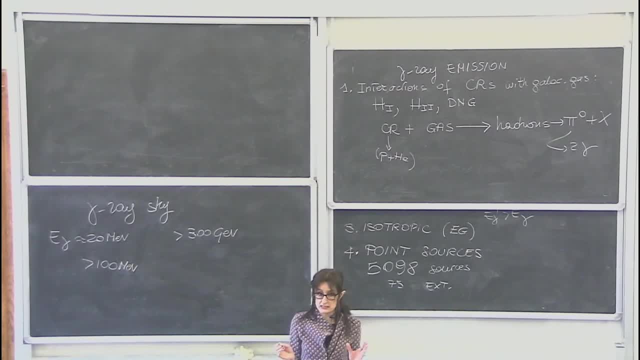 but the telescope can detect and can resolve an extension. The biggest extended sources are indeed, let's say, structures. One of these is the so-called Fermi bubble that has been detected a few years ago, And these are enormous structures across the galactic plane. 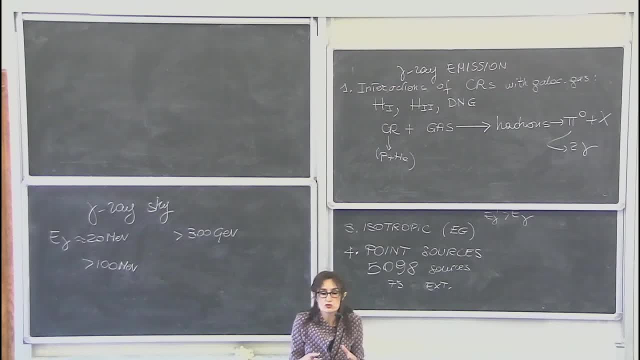 There is another big structure, which is called Loop 1.. And then there are sources, astrophysical sources, that have been detected as spatially extended. Many of these sources are linked to active galactic nuclei, in particular the galactic nuclei of the Milky Way. 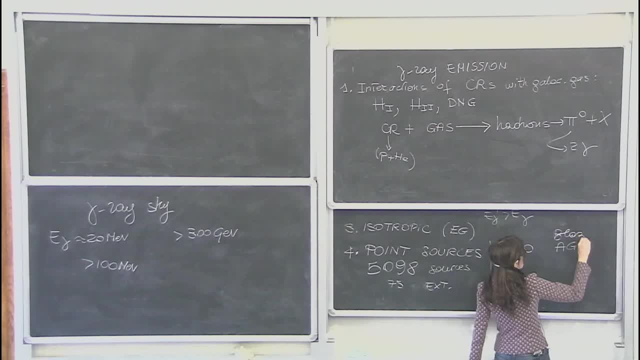 In particular they are blazers And of course, these are all extragalactic sources. A number of sources- which is pretty high, it is 241, has been measured to be pulsars, which is one of the big results of the Fermi Large Area Telescope. 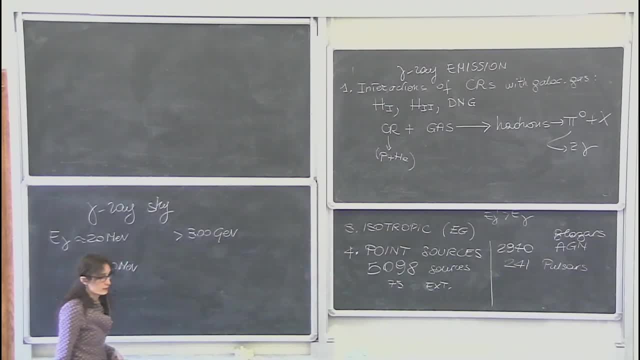 to have measured an incredibly high number of pulsars With respect to the state of the art. And there is another point that I want to underline: in this catalog There is a number of sources, which is about 1,500, which in the vocabulary of astrophysicists, is unassociated. 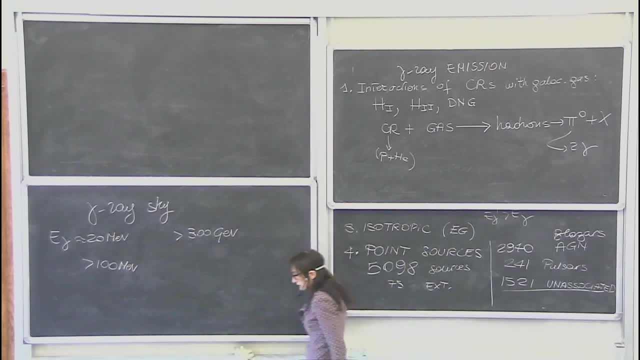 These are particularly interesting sources. Unassociated means that they have no counterpart at any wavelength. Usually one points a source and finds an excess and is sure that there is a source there And immediately people look at catalogs, mostly at radio catalogs. 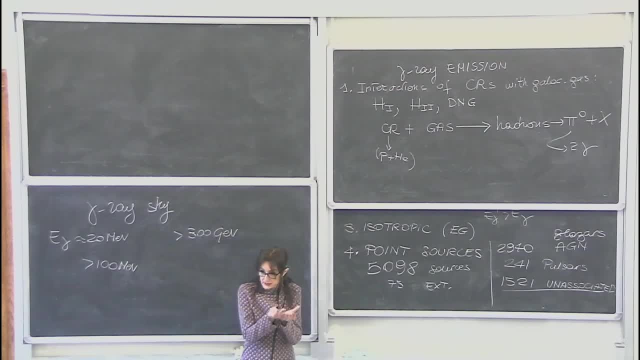 to see if, in the same place of the sky, somebody has seen a source and this emission, for example in the radio wave, is compatible with what people are measuring in gamma rays. Well, there is a significant fraction of sources that at the moment is not associated to any radio X-ray visible or whatever wavelength. 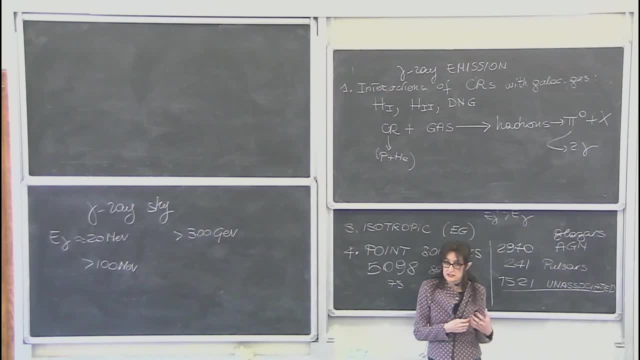 And now it's happening that people measuring gamma rays or unassociated gamma ray sources are asking to colleagues working, for example, at radio telescopes to look in that precise portion of the sky to see if, looking with more detail and knowing the position, 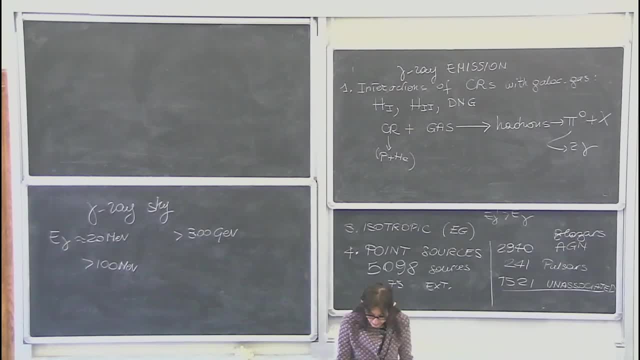 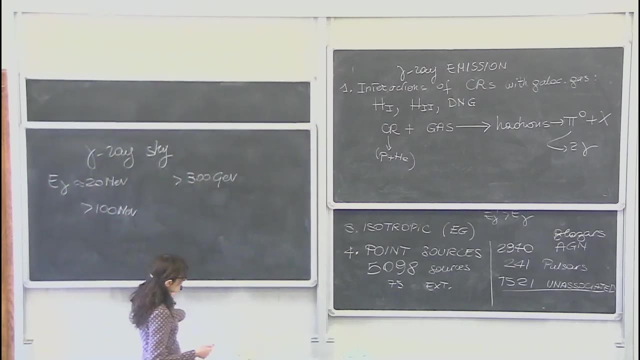 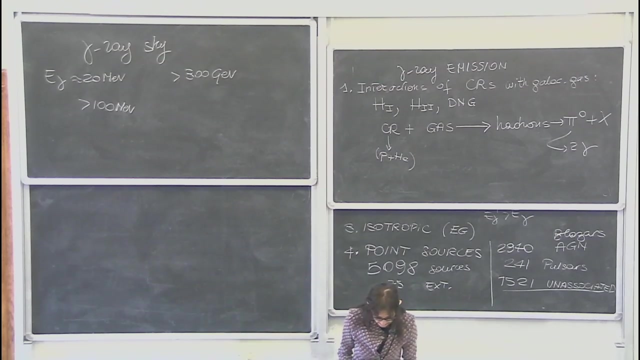 this source is possible to see. This is really a big and very interesting multi-wavelength interaction that has been improving Since these catalogs among different astrophysical communities. Then I don't want to, So let me come back. So we have point sources. 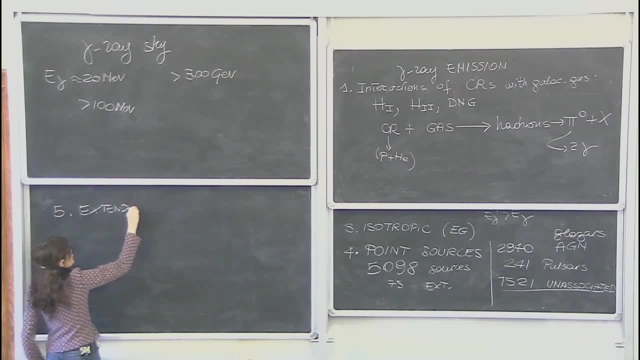 We have extended sources that if you want to predict the gamma ray sky must be put in a very different way when you try to predict the Fermilab sky. And then there are some residual photons from the Earth and the moon limb. 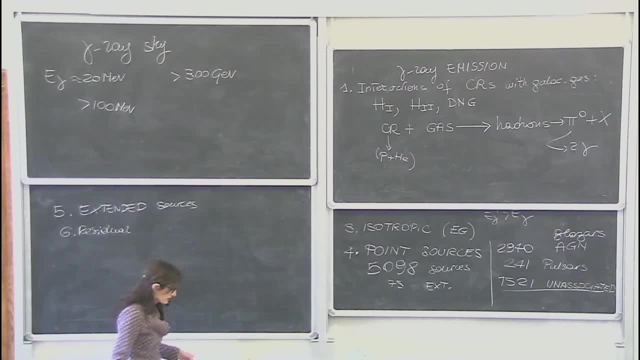 but they are not very relevant above, let's say, 200 eV. So they in many analysis they are modeled or they can even be neglected. So you see, we have the 0.1 emission, which is fully galactic. 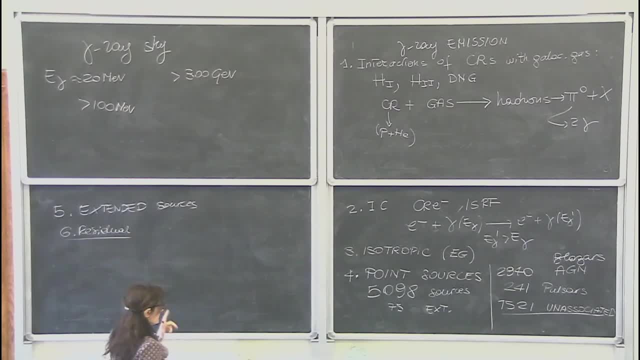 The second one is again fully galactic. The isotropic is very likely extragalactic And point sources it depends. Pulsars are mostly galactic, KGN are extragalactic, Extragalactic The first two emissions. 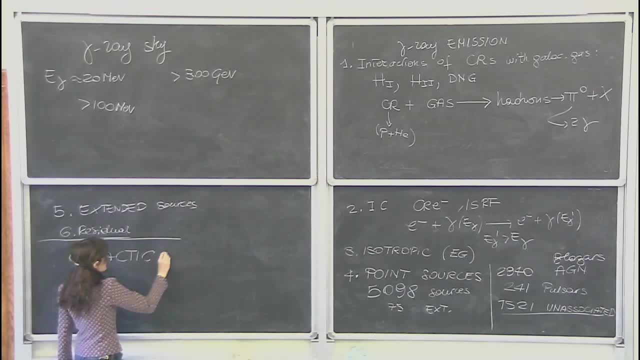 are composing the so-called galactic diffuse emission, which is a kind of sea of photons produced by all the scatters of cosmic rays on the gas and on the interstellar radiation field. This galactic diffuse emission is dominant, And it is dominant almost at all latitudes. 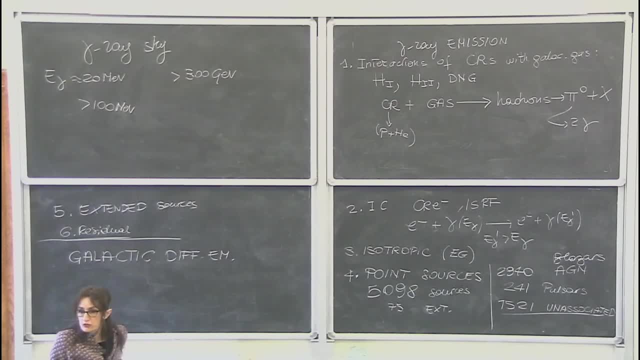 Of course, going towards the galactic plane it is overwhelming. Going to higher latitudes it is less, a bit less relevant, But it is almost everywhere- at least 50% of the photons that you measure in the sky. So if you are interested in studying the galactic diffuse emission, 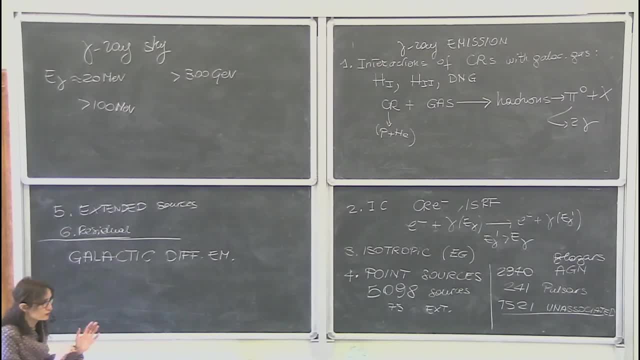 well, it is almost everywhere, So one has a lot of places to try to understand it. But if you want to measure anything else, for example some possible dark matter annihilation or studying astendic sources or anything else, it is well not really a background. 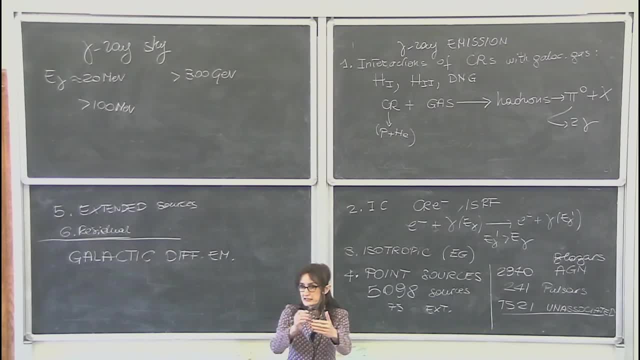 It is a foreground, because between you and any other source there is always this thickness of photons that you cannot avoid. There is no way to subtract this foreground, So the only way that physicists have to deal with it is to model in the best way. 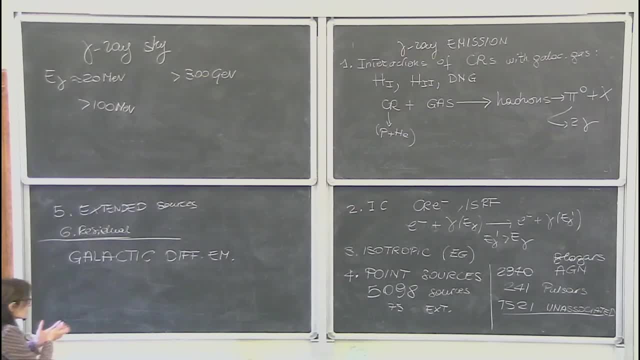 and then to put it as a template or do all the other analysis with some assumption about the galactic diffuse emission. So the galactic diffuse emission is cosmic rays And these cosmic rays are proton, helium and nuclei. The target can be the gas. 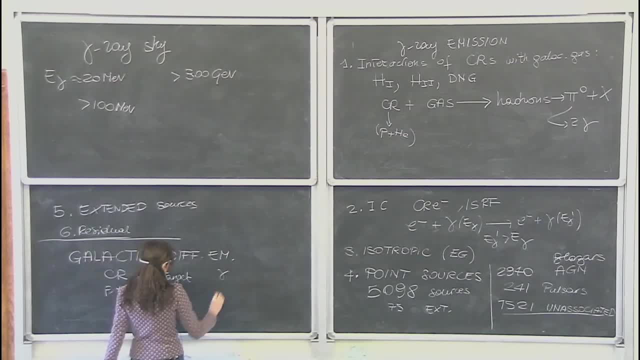 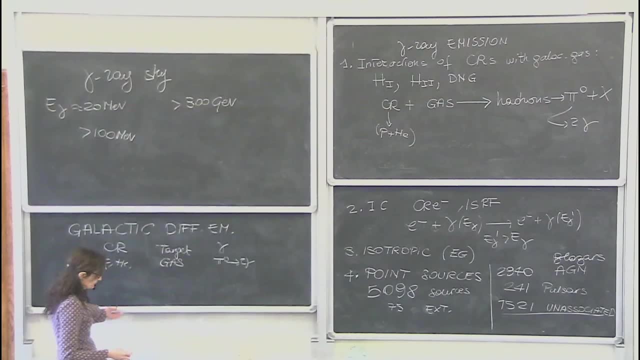 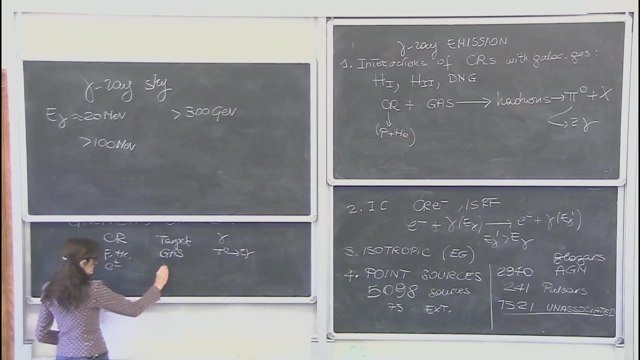 And the gamma rays in this case are given by pi zero, decay into two gamma, Or the sources are E plus, E minus that interact on the interstellar radiation field and give photons via inverse Compton. There is also well, just to 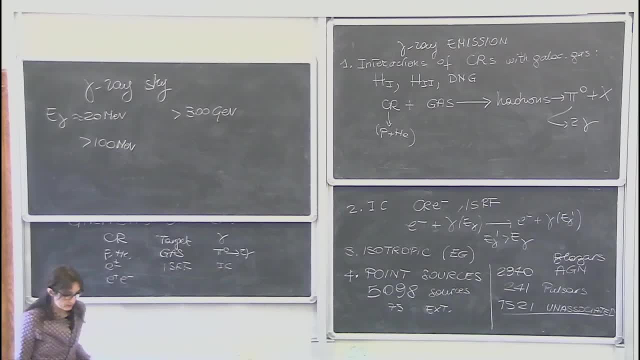 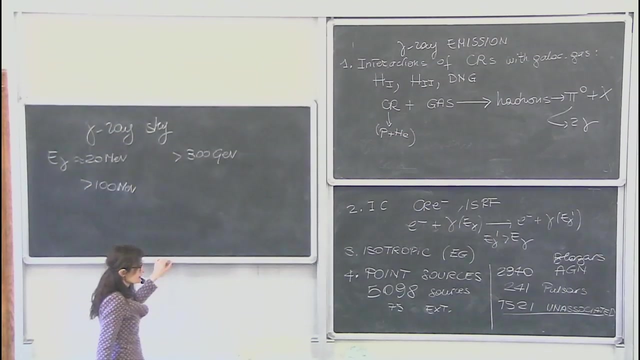 For completeness I put it. I didn't spend time on that, But I mean you can easily recover the physics of this. There are also electrons that can interact on the gas and give photons via Bram Stralung. So in order to predict the galactic diffuse emission, 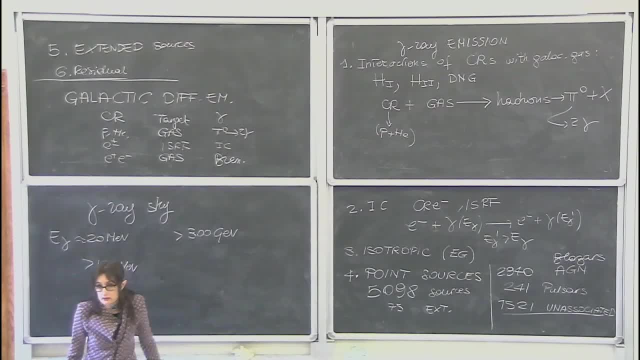 or to determine the galactic diffuse emission. one should, in principle, perfectly know the cosmic rays And the cosmic rays in every point of the galaxy. we only have detectors at the Earth, So we should know how protons are behaving. for example in some spiral arm of the galaxy. They are not necessarily the same flux as we measure here. We must know the distribution of gas and we must know the interstellar radiation field. So it is a big work to arrive at a determination of the diffuse emission. 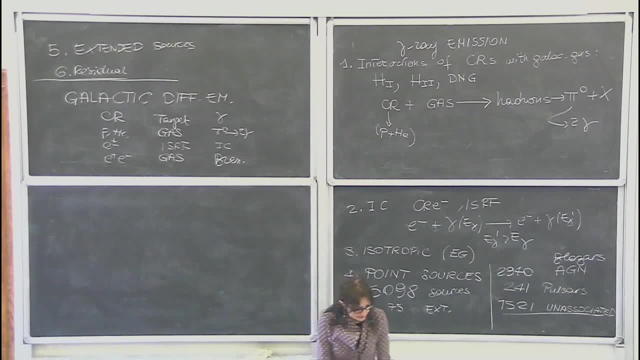 the gamma ray diffuse emission. The gas comes under the three forms H1, H2, and also the molecular hydrogen. So this is neutral atomic. This is ionized, which is a fancy way to say that it is protons. 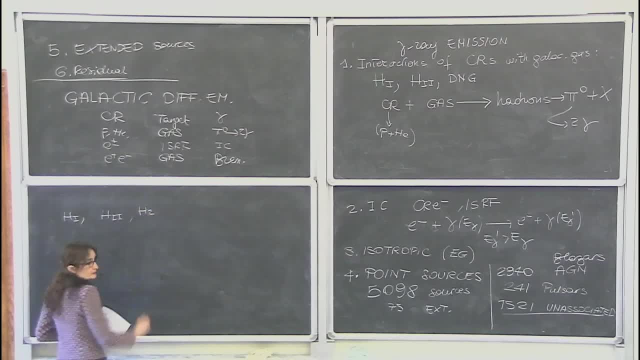 And there is molecular hydrogen. This gas must be measured in all the places of the galactic plane, or where it is anyway, also out of the galactic plane, And there are very intense and very difficult surveys that try to measure what we call the column density. 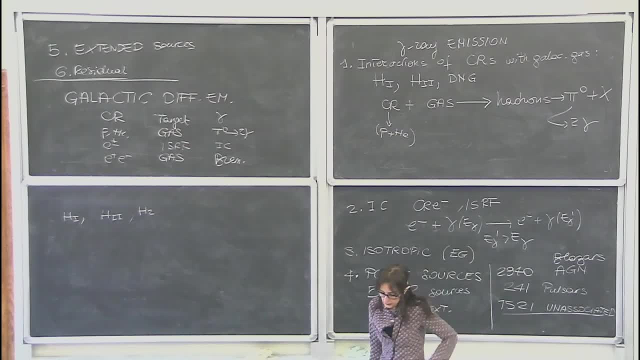 of the gas along the line of sight. Moreover, the gas comes at different temperatures, So, according if it is cold, if it is warm or if it is hot, the physics is different and also the measurements can be a bit different. 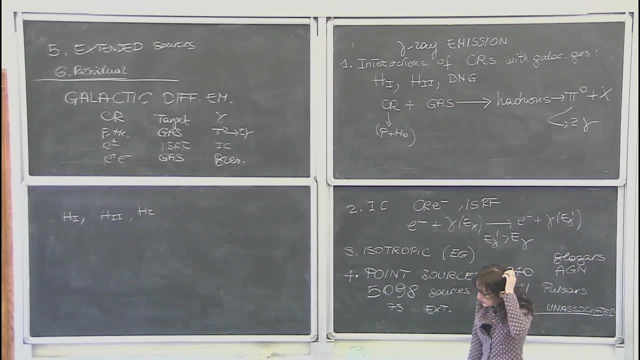 There are some more notes that you can find here if you are interested. Just what I want to say is that one of the most interesting tools to measure the gas, the distribution of gas, is an emission line which is very important in astronomy. 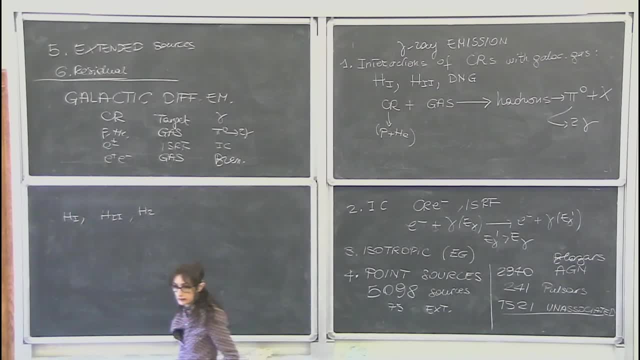 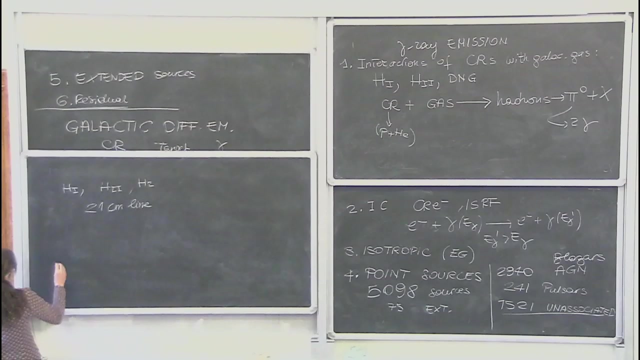 and which is called the 21-centimeter line. And this 21-centimeter line is connected to this quantum mechanics transition in the hyperfine And this is the structure of atomic, of each atom. So it happens when the atomic hydrogen. it is in the fundamental state, but the spins of electrons and protons can be weather-aligned, weather-opposite. So there is a splitting of the energetic states of the atom and the splitting between two states is of about 6, 5.9,. 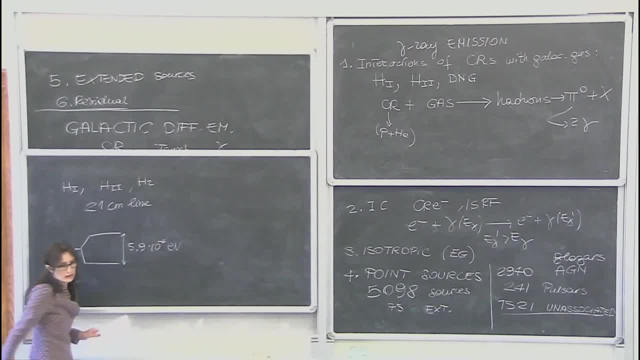 10 to the minus 6 electronvolts. This is really hyperfine with respect to the energy levels of hydrogen. And this is when the spins are aligned and this is when the spins are opposite. So the upper level when the spins are aligned. 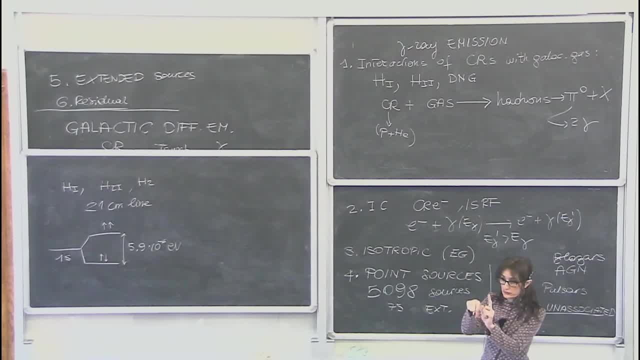 can go to the lower level when the spins of protons and electrons are opposite, emitting a photon. So the stabilization of the quantum level comes with the emission of a photon, And this photon, with this energy, has the frequencies, the corresponding frequencies. 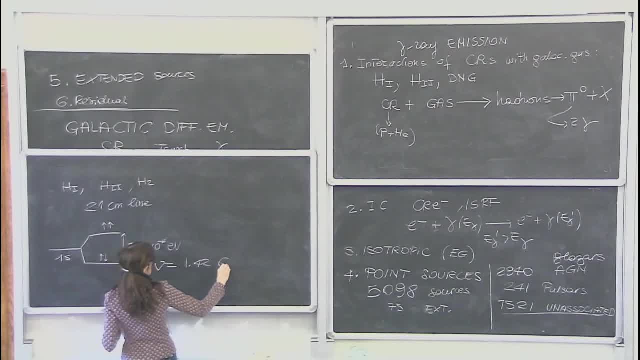 of 1.42 gigahertz, which is radio close to microwave And the wavelength is 21 centimeters. This is why these 21 centimeter surveys are named. So with radio telescopes that can make deep survey, one can reconstruct. 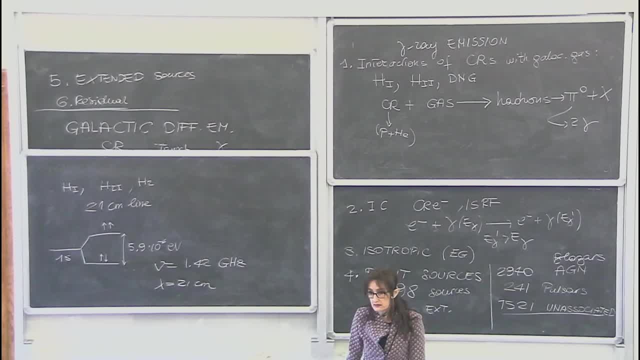 can reconstruct the column density of gas in, let's say, in the galaxy, And you can imagine yourself that it is not a trivial task to have a map of gas for all the galaxy And for all the three states of hydrogen and for all the temperature. 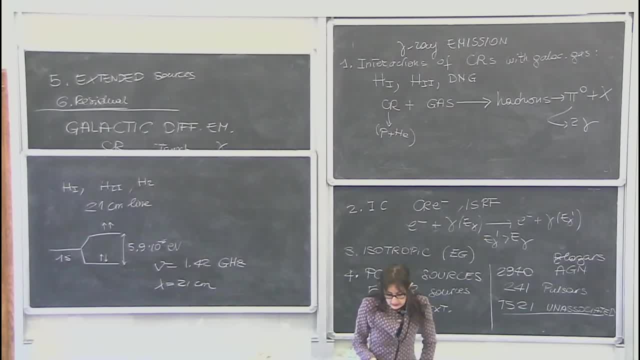 it comes with. Some other lines are measured. For example, measuring the molecular hydrogen is not possible via this way, But people measure another transition, which is the transition of carbon oxy oxide, how to say. And there is an emission line of this molecule. 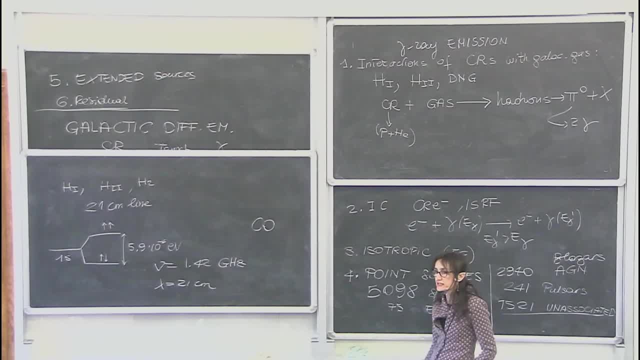 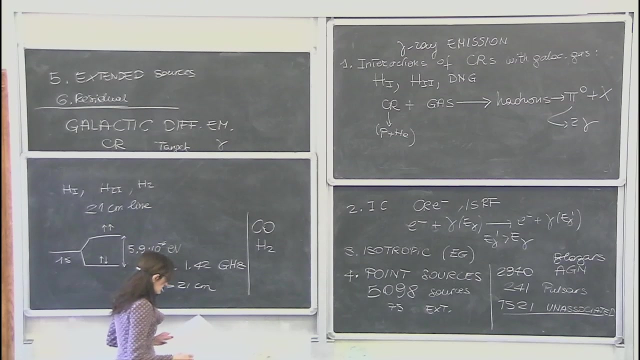 And this molecule is very often associated to the presence of H2. So the emission of CO is a tracer for the distribution of molecular hydrogen. This line for the emission, the emission of CO, is at a wavelength of 2.6 mm. 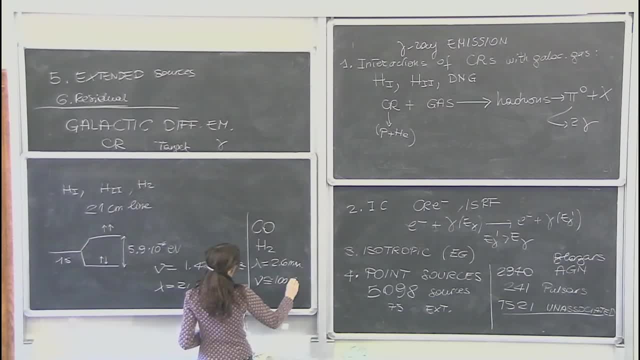 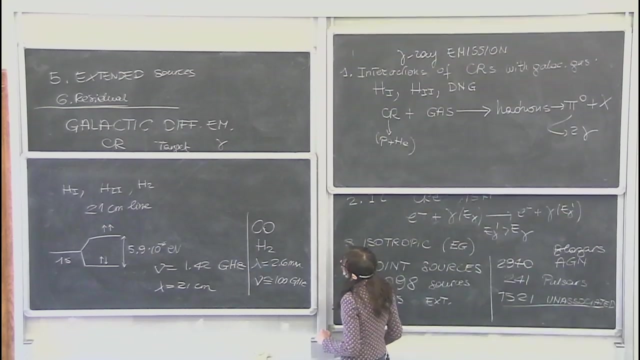 that means a frequency of about 100 GHz. So in the lucky hypothesis in which our colleagues working at different wavelengths and studying also the interstellar radiation field provide us with map for any component, we can hope to have a prediction for the galactic. 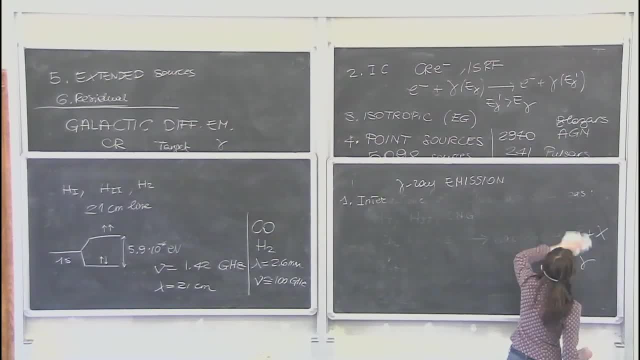 diffuse emission. So since, as I was telling you, the galactic diffuse emission is unavoidable and it is a foreground for any measurements, what people, in particular the Fermilab collaboration, has done is the following: Well, it is too. 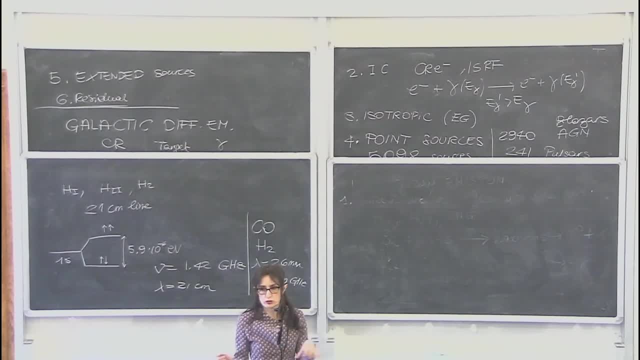 it is impossible to predict the diffuse emission in all points of the galaxy because we don't know cosmic rays everywhere, or at least it is difficult. What they did is to have maps for the gas, for the interstellar radiation field and try to make hypotheses also for all. 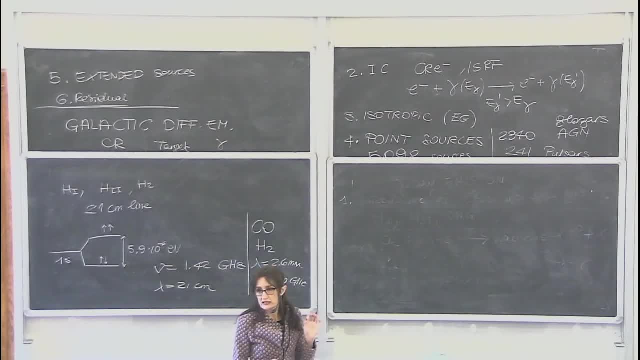 the other components and to make a prediction for the entire sky. So the idea is to predict the whole gamma ray sky. This is, of course, a prediction which is a function of latitude, of longitude, latitude and energy, And it needs 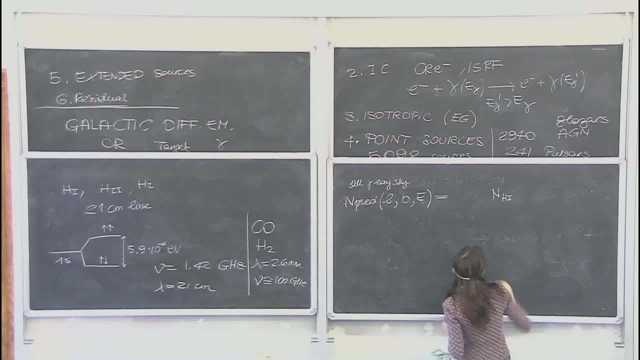 the distribution of H1.. And the distribution of H1 is a function of coordinates, And there is a factor in front of this distribution which is a function of energy, and it says how photons, and at which intensity and at which energy are produced in any point. 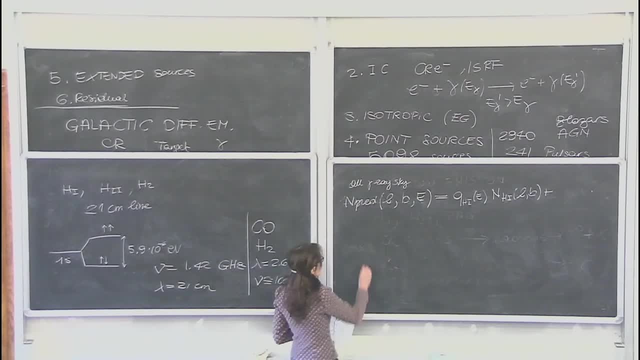 where we have this gas. And then there is the same structure. This coefficient q is called emissivity for any of these components. So there is CO. The column density is called W for CO, and it traces mostly molecular hydrogen. And then 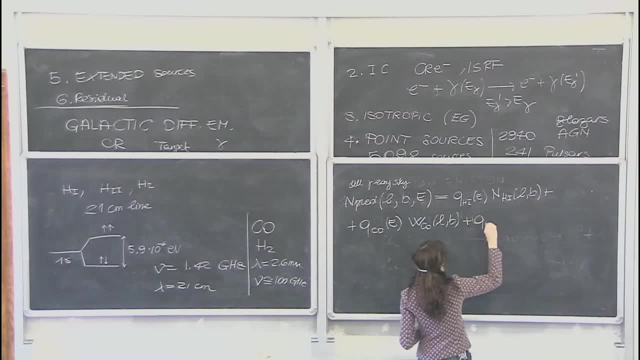 there is a similar emissivity for the dark neutral medium, whose determination is even more difficult than the previous two ones. You can read- there are some papers on that if you are interested- And this is the dark neutral medium which is again convolved with this. 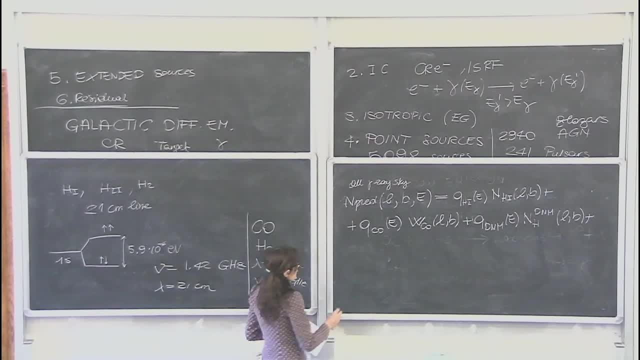 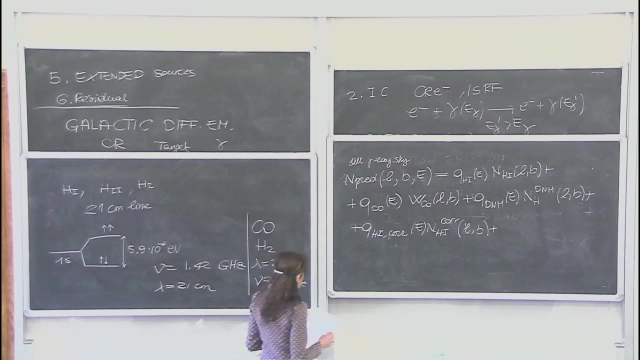 spatial distribution. Then there is a term that I don't want to. I just put for completeness, which corrects somehow the distribution of H1. Just take it for granted, because otherwise times runs. You can take the Fermi paper to the components that we 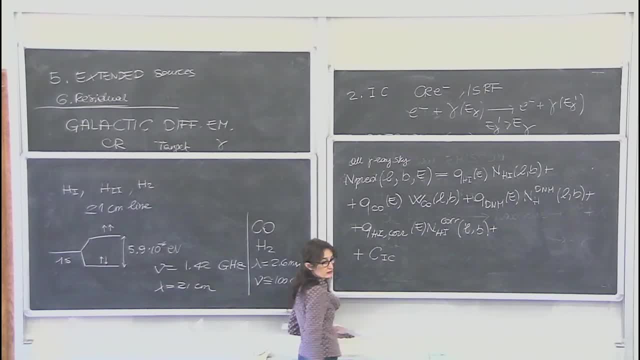 have studied better in this course, which is the inverse Compton, And this is the inverse Compton normalization factor. It is a function of the energy and it is convolved with the maps for H1.. This comes with an energy because it is ultraviolet. 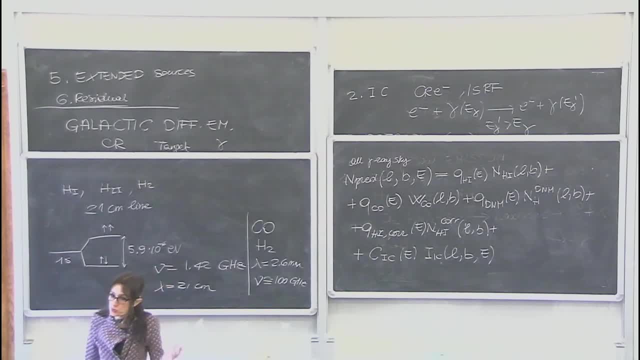 it is visible, it is infrared and it is the CMB. So you have a distribution on all the wavelengths which is different. Then one should predict we should make a distribution which is not point-like. And then there is the isotropic distribution. 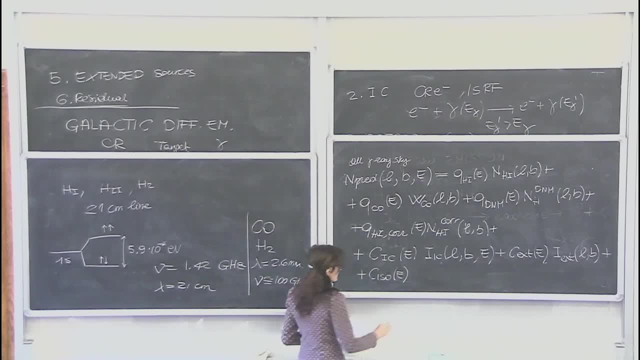 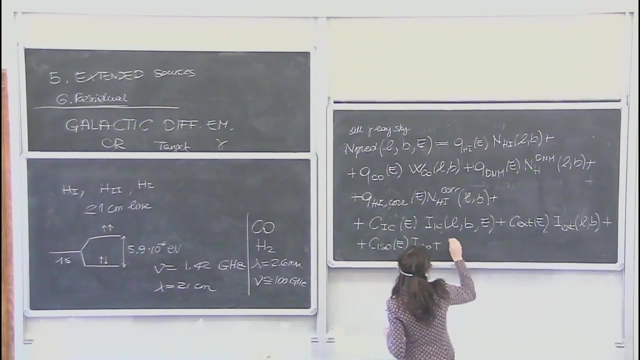 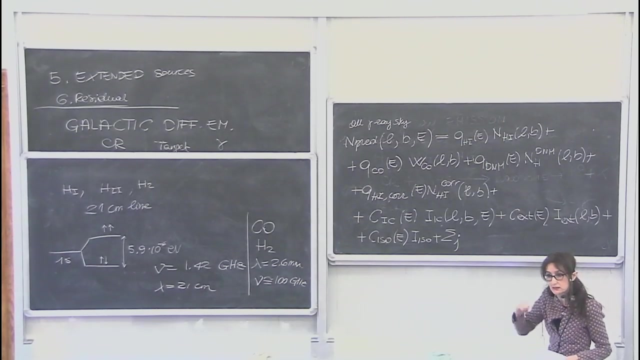 I told you before, which is a function of energy and which is preferably determined at high latitudes and low latitudes. So if you have a full sky prediction, put a kind of free normalization to let it vary to better fit the all gamma ray sky. 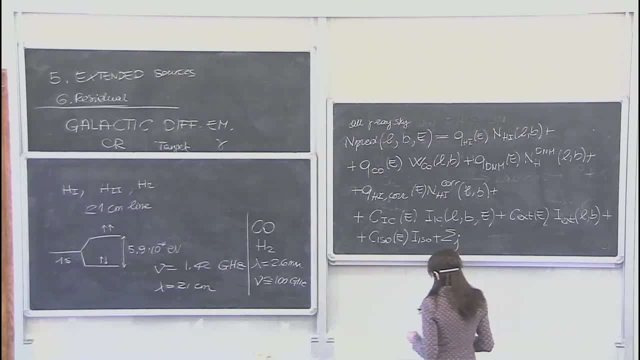 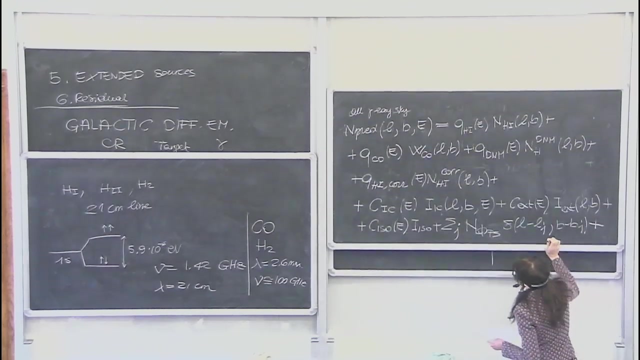 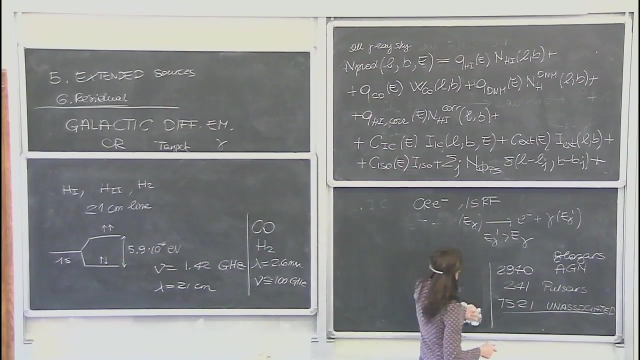 And then there are the point-like sources. The point-like sources are a flux and they are located in a precise position of the galaxy. So this is j and this is b minus bj. And then I don't add, we have much less relevant. 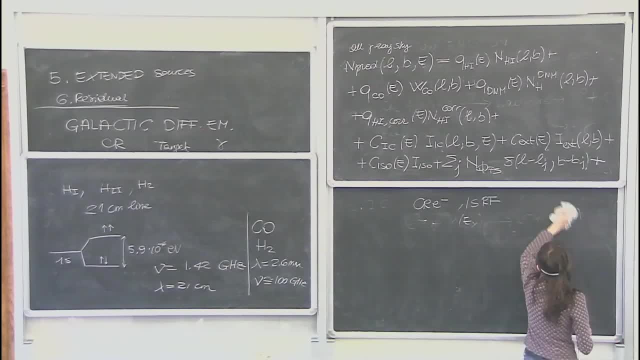 There are some photons that hit the detector and that are given by the earth limb, And some contribution, that one that come from the sun and from the moon. Okay, So this is the full way to write the gamma ray sky And what people usually 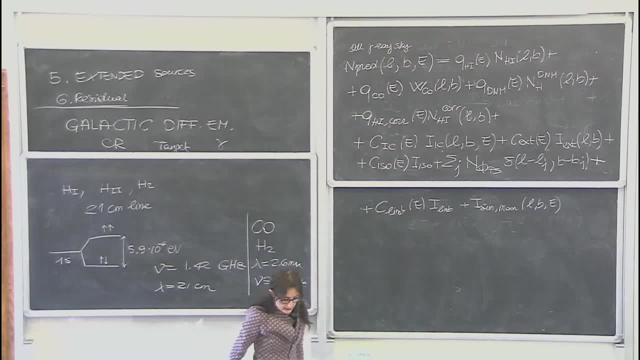 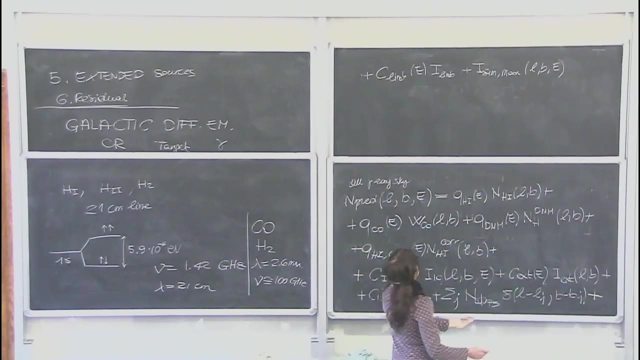 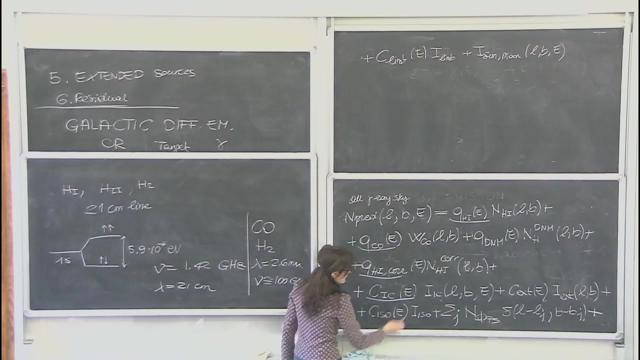 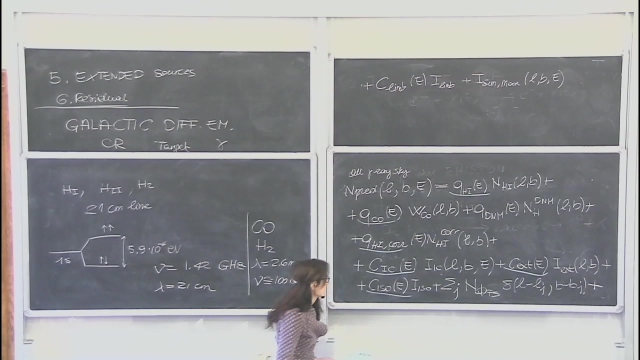 do is that, well, this, all the other components have the emissivities or the normalizations, let free. So emissivities are one, This, this is the normalization for the inverse, for the extended sources And these sources, let's make the hypothesis that this one detect. 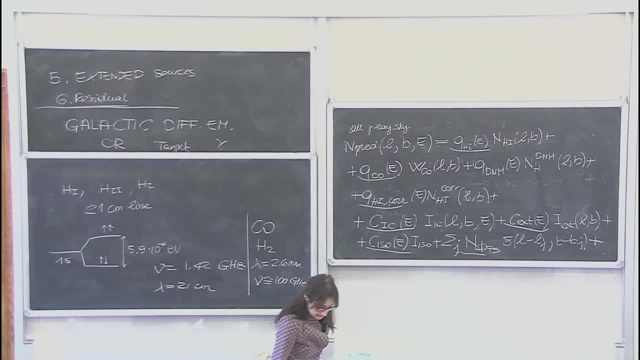 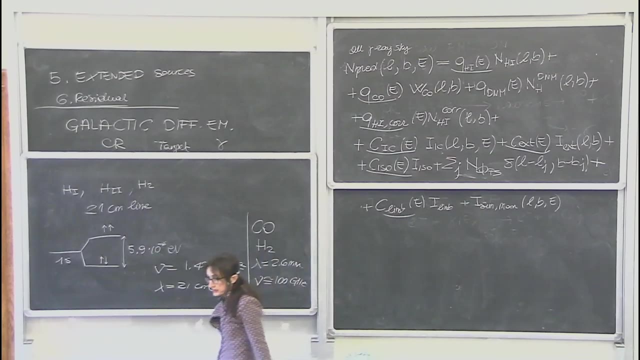 them are more or less known, but one can leave the normalization of the flux of point sources also to vary. So what we are doing, and have done in the past, and also some other collaborators, is to fit all the sky and to give results for all the. 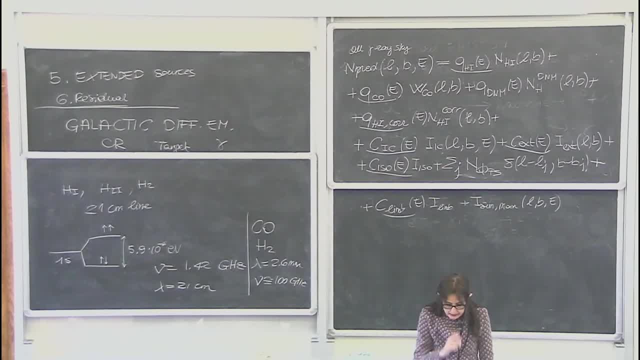 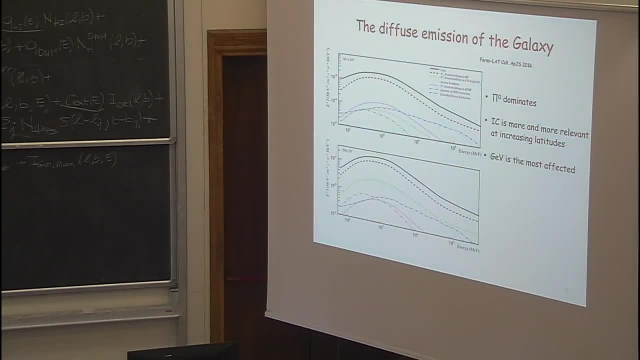 precise results, And this is one of the results that I wanted to show because it is, I think, understandable with the tools that we have developed together this week. These are the results of the analysis of the galaxy plane. This is the latitude, so 10. 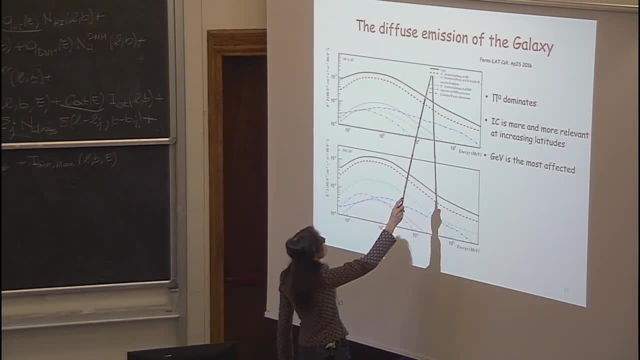 degrees out of the galactic plane, so from 10 to 90, and this is around the galactic plane by, and you see that at high latitudes it is dominating the sky. And then there is the second component, which is this light blue which is 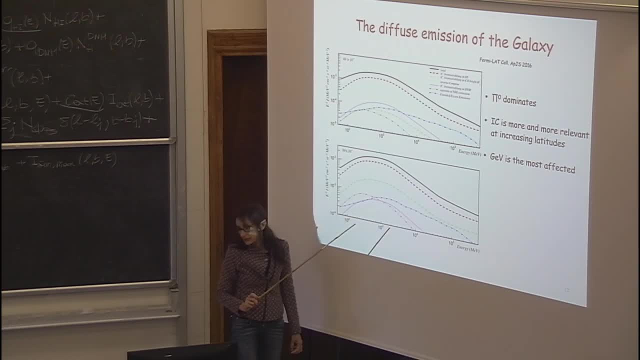 emission. So let's concentrate on these two components. Look at the red and the green is for hydrogen H1 and the green is for molecular hydrogen. So they have splitted even on these two different targets. But you can see that the red is for 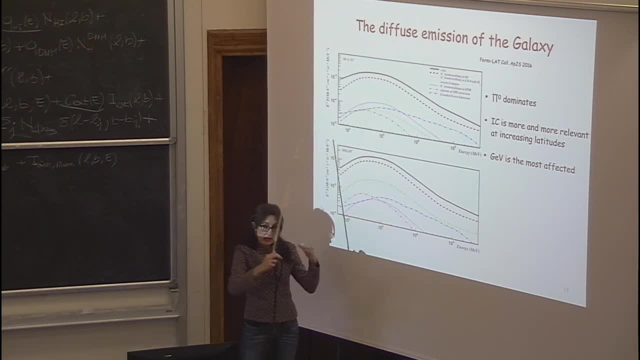 the hydrogen and the green is for the hydrogen. So the red is for the hydrogen and the green is for the hydrogen and the green is for the hydrogen. So you can see the red is the hydrogen and the blue is the hydrogen And the green. 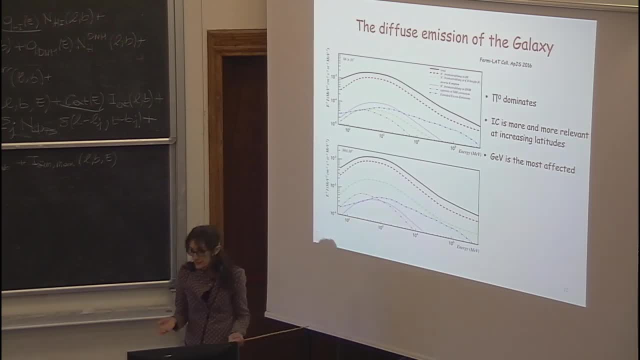 is for the hydrogen, So if you, your resultant must be included. okay, this is what I wanted to say. you see, also the energy dependence. the energy dependence, dependence of this component components- is pretty well not the same. but the place in which you have the most of the photons is in the GV region and this was visible also from the maps that. 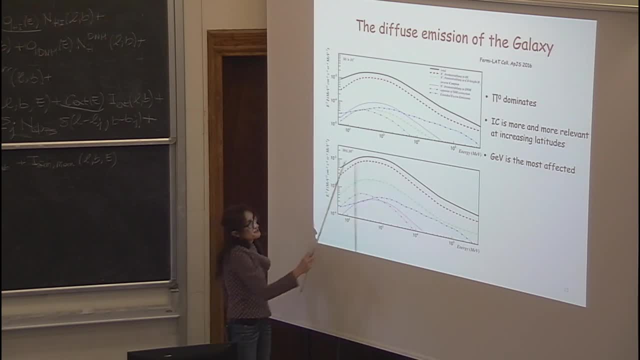 I showed you before. so from one side it is the privileged place because you have you have a lot of photons, but you must be careful to very well model your galactic diffuse emission because it is in an avoidable foreground. good, so this is more or less. 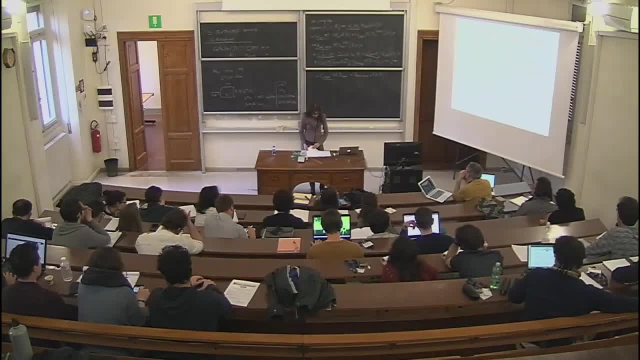 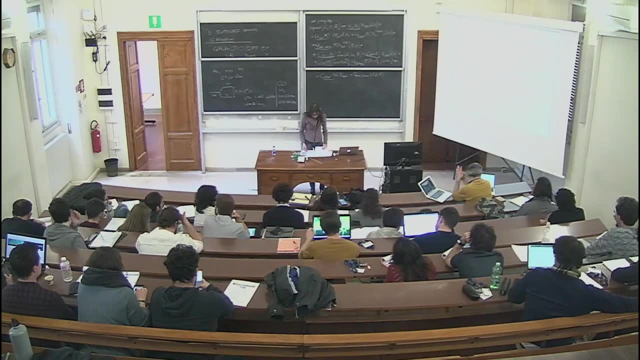 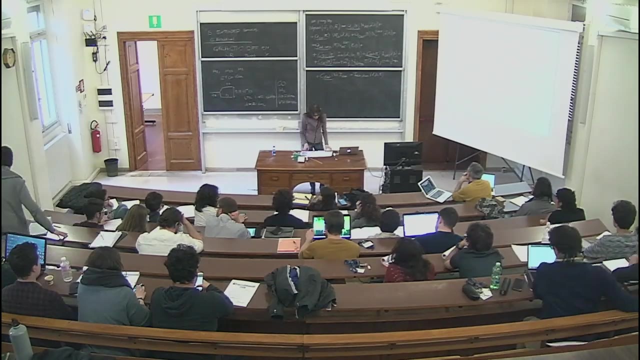 you can see that the energy dependence of this component is pretty well not the same. so this is more or less what I wanted to say about the gamma-ray sky, and now, given the relevance of this, cosmic rays, I come back to what I started to discuss. I 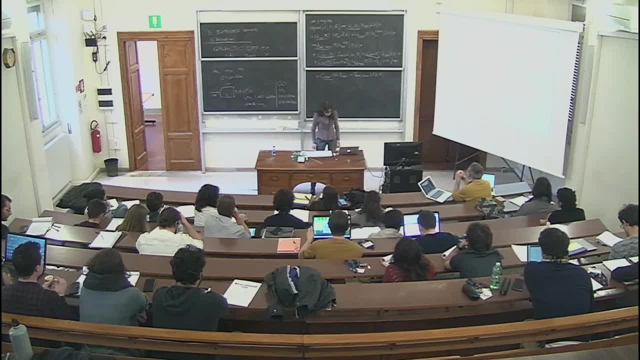 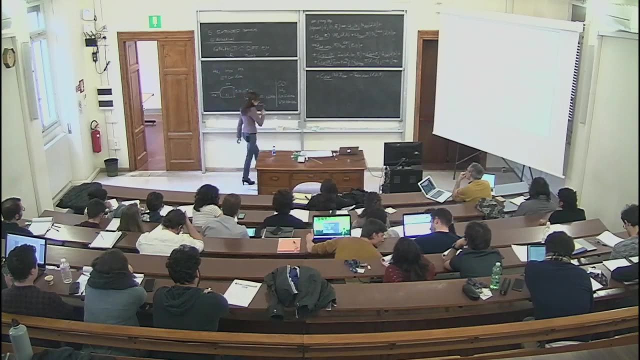 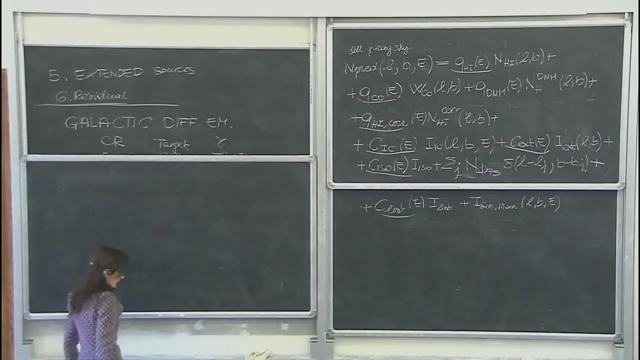 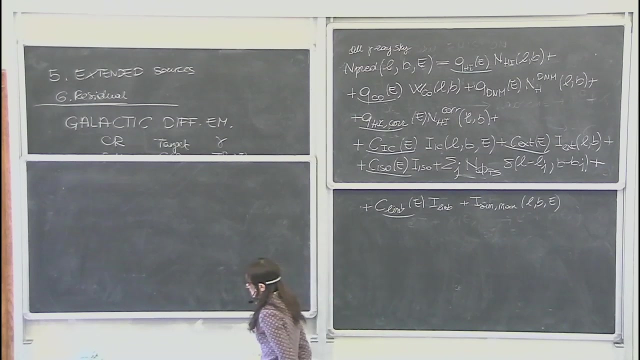 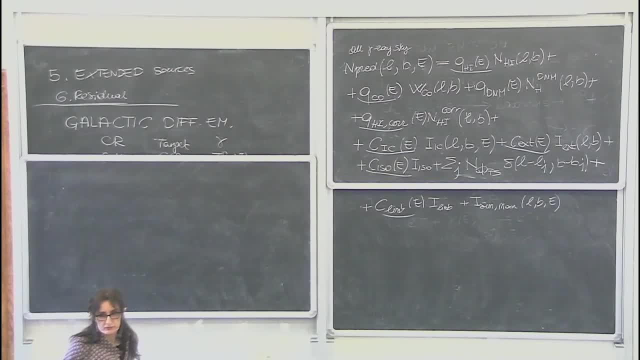 again to our transport equation, the transport equation. now you understand what it can mean to solve the transport equation in every point of the galaxy. it is would be relevant that it is a really a difficult task. so let's come back to spend a few words about sources which are typical of secondary nuclei, For 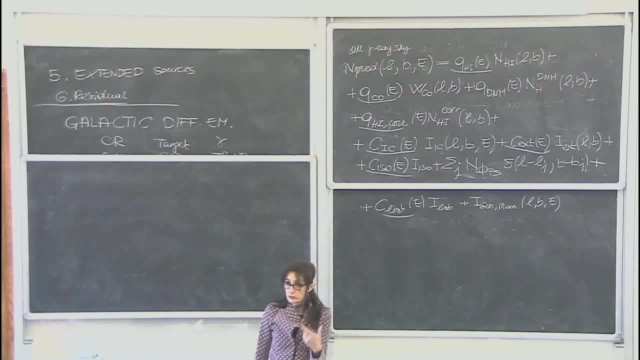 primary sources. we have seen supernovae. we have seen pulsars. you have done some more learning on Tuesday afternoon. you have seen dark matter. These are the possible primary sources that we know, And then there are sources giving secondary nuclei, And secondary nuclei are really a valuable means of 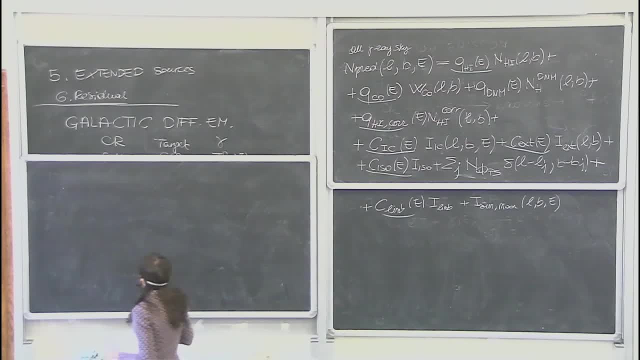 information in the galaxy. So now let's come back to charged cosmic rays and to secondary nuclei. So let me write in some more details how the distribution function for a secondary nucleus is different from the distribution function for a secondary nucleus. So the distribution function for a secondary nucleus is given when a nucleus I 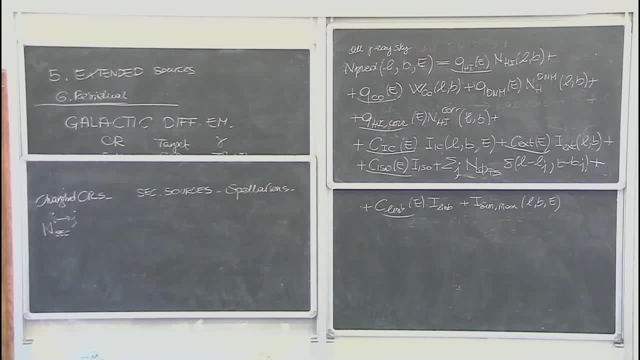 produces this very nucleus J. This can happen at different energies and at any place in the galaxy. I avoid here a time dependence. usually these sources are steady-state, We can put it, but it is for special cases. In order to compute this term, one must sum. on all the nuclei I, which are the cosmic rays that can make a spallation reaction. Then we have to sum on all the species of the interstellar medium And we have to compute a convolution from a minimum energy, which is usually a kinematic threshold. let's say: 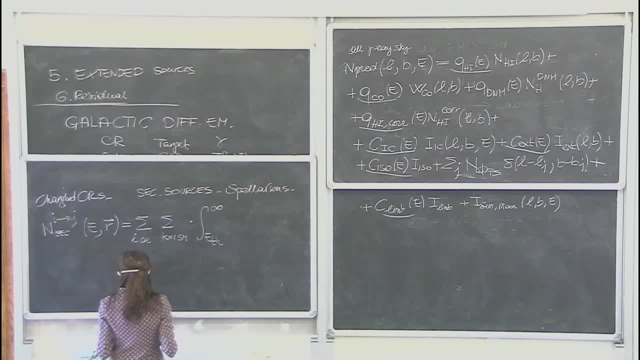 in principle to infinite of the Ni nucleus. So I have a solution for the. So let's have a solution for the nilion-nitral of the nucleus times. the clock session of the nucleus i over the nucleus k, where the, then we have the velocity. I put P, but it. 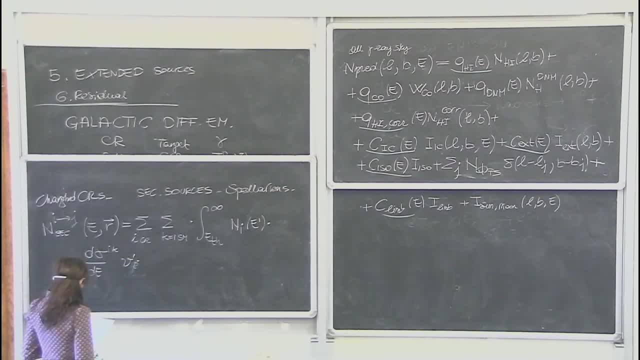 is I. and then we have the density of the interstellar medium, which is given by different species. I see now that in my notes I forgot density- sorry- of the interstellar medium. so in order to compute this class of nuclei, you have to know the cosmic rays, flux, the distribution of the gas and a full set. 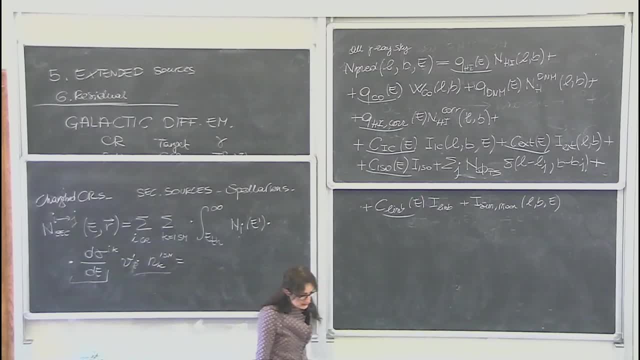 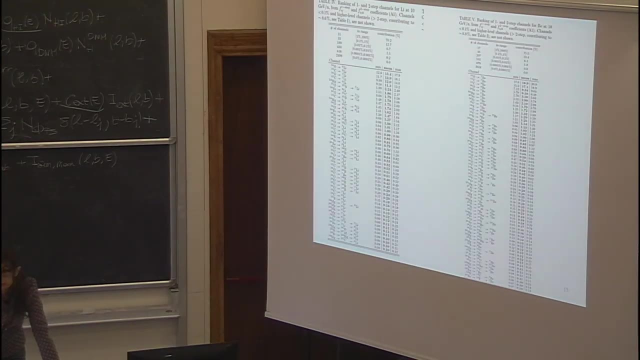 of croc sessions. I was already hinting at this problem, and now I'm going to show you how to do it. Now I have some- what is it? some figure. so you are not, of course, required to read this figure, it is just for your emotional reactions. I have to say, This has been. 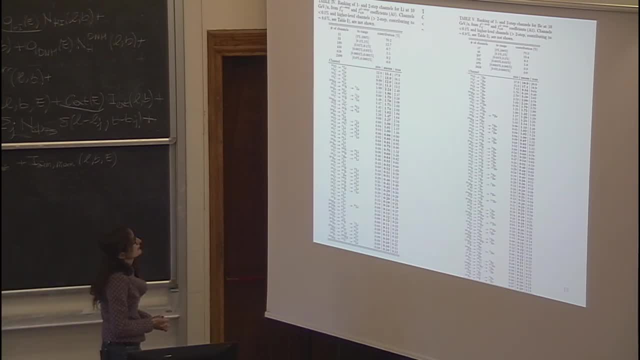 taken by a recent paper, and on the left side of this figure, these authors have listed all the possible reactions that occur in the galaxy and that produce lithium. So you say, okay, nice, now AMS has measured the lithium flux. I want to predict it. Well, it's nice, but it is a huge work. 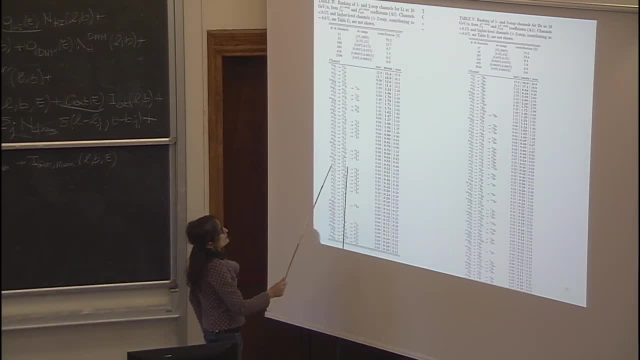 These authors have also somehow ranked the relevance of each contributions or some part. you can decide to stop adding contributions, But this is just to tell you, to show you, that this physics require not only to know the flux of oxygen-16, of silicon-28,. 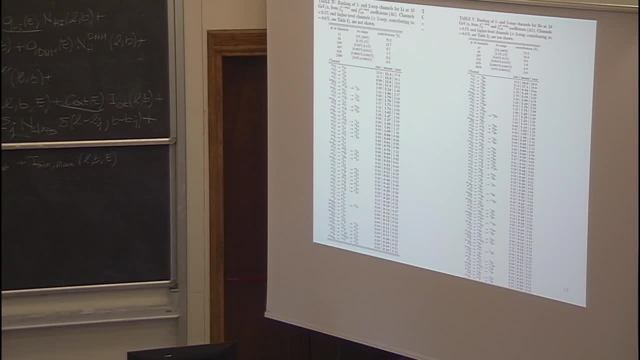 but you must know the cross-sections and the only way is to measure them at colliders. So this is the physics, really, that needs multivariate length and multi-messenger and multi-disciplines inputs in order to perform it, and to perform it with. 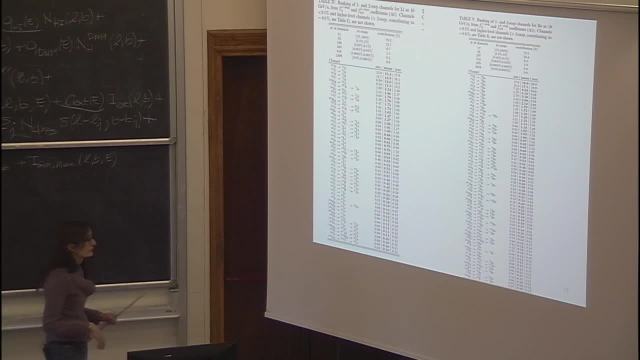 precision, because now data from example, from AMS and first also from Pamela, and there are other experiments, is pretty precise and the data are provided with few percent of errors, which is very similar to the precision of ionic physics. so we cannot say okay. 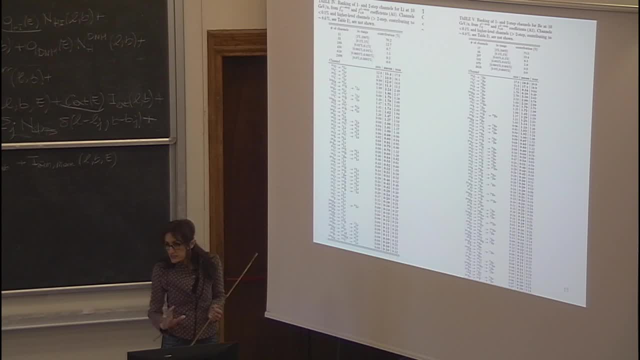 I make some approximate. it is no longer possible. otherwise you missed the interpretation of some data point, And this is the same as before, but this time from the radium. so you see that there are really a huge number of reactions that should be included. 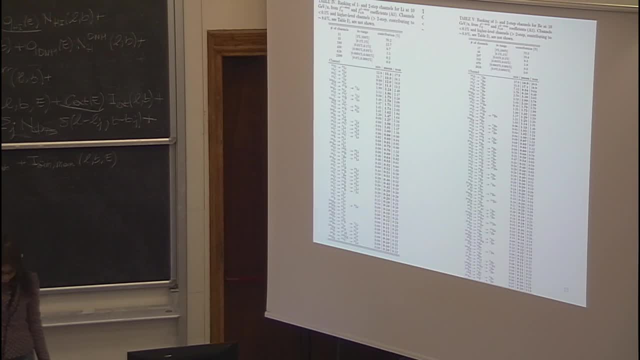 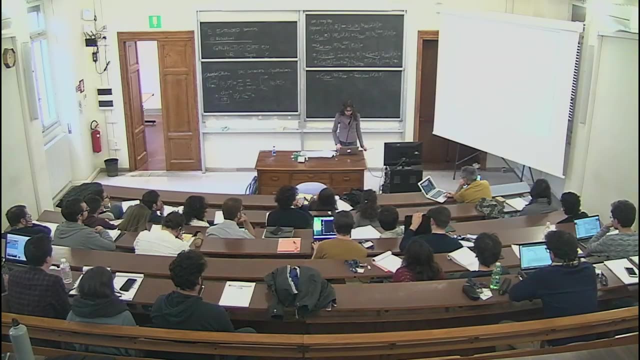 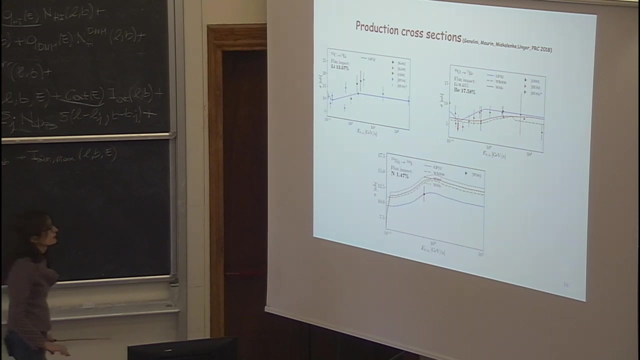 to be at a very, very precise level of prediction. Maybe I have other two figures that I show, So this is a very, very precise level of prediction. This is a typical work that people doing clock session analysis are forced or so. 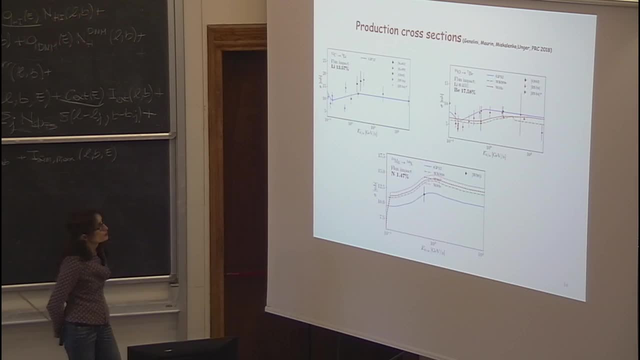 these are taken from the same paper as the huge tables. The aim, my aim, for showing you this figure is that, well, there are some analytical models for this is, for example, the production of lithium-6 by carbon-12, and you see that we have some data, but even it's not. 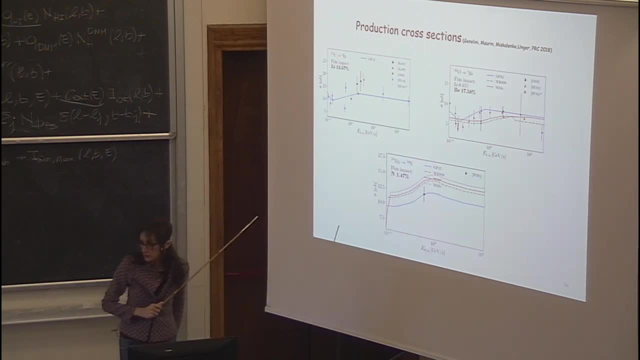 really a clear situation from an experimental point of view. But for example, here the production of nitrogen-14 by Mg-24 has one data point. And then, well, you try to fit, you try to fit, you try to fit. 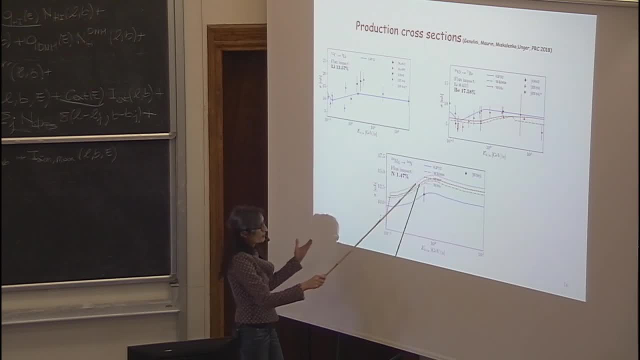 you have some extrapolation for previous empirical models, but it's far from an easy task, And the uncertainties that this kind of physics brings to the prediction of secondary nuclei is often huge, And in the last years it has become one of the most important. 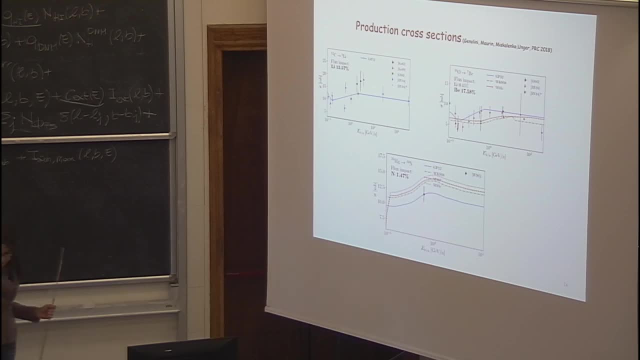 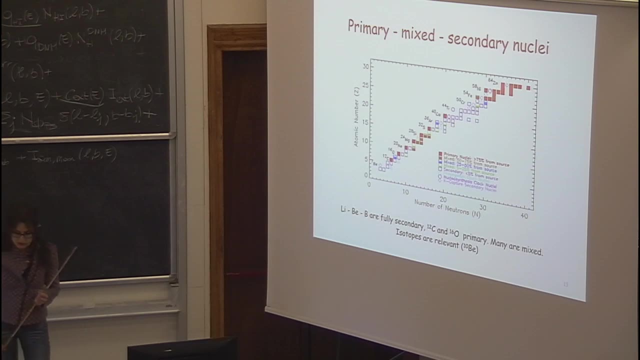 sources of analysis. So this is an example of uncertainty. Maybe it was before, yes, Now let me show you this figure. This figure is kind of a summary of the different possible sources that we have in the galaxy. This is the atomic number and this is the number of neutrons. 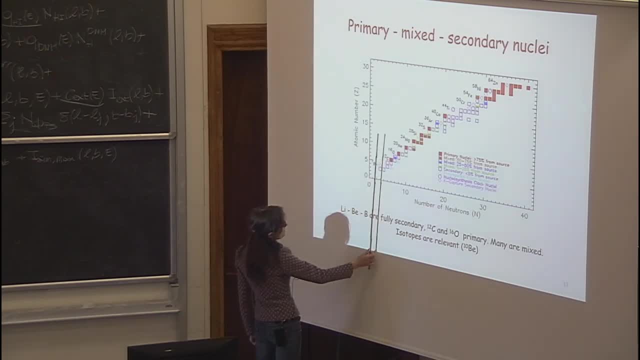 That means that here you have a species, a specific species, for example beryllium, with different isotopes. Okay, so a species can, species can come with different isotopes. So take a nucleus that you like I don't know. 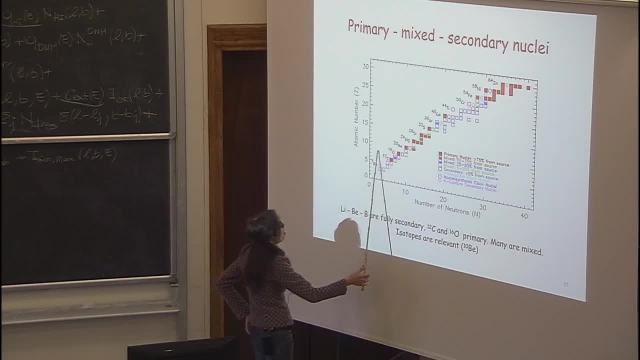 We can, for example, consider oxygen which is eight Z equal to eight. It is mostly primary. Full red means that at least 75% of oxygen- 50%- is from sources, so from supernova remnants. But there is, where I am here, some secondary left. 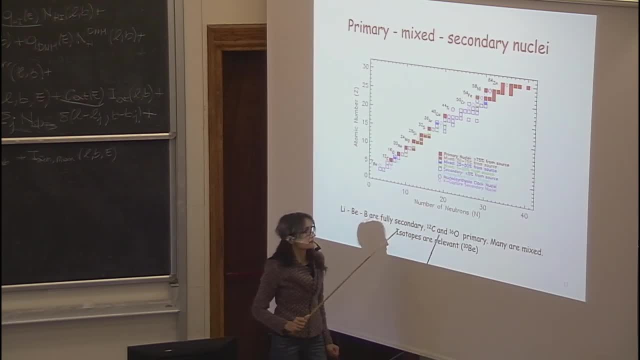 which is anyway less than 5%, which is not very relevant. And there is another part which is mixed, mixed between primary and secondary, which is not so, let's say, easy to separate. For example, take lithium: Lithium is here. 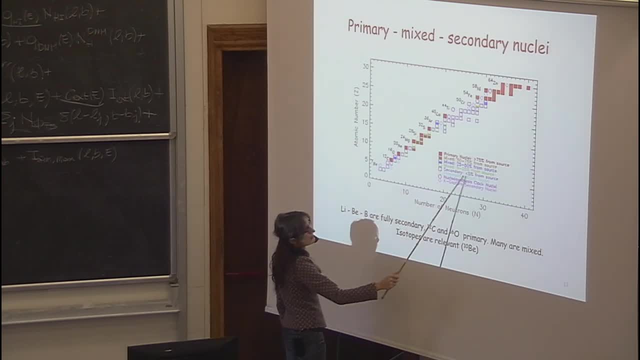 Lithium has two isotopes and these two isotopes are fully secondaries, And so come back to the cross-section problems. for this kind of nuclei. There is carbon. There is carbon. Carbon is mostly primary. It has a small secondary component. 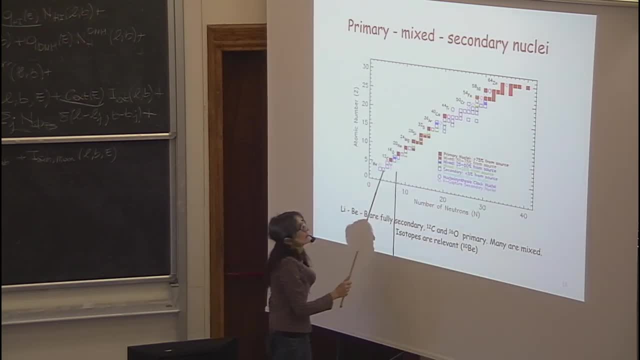 given from the spallation of higher nuclei. And there is, you probably know, by other ways, the 14-carbon, which is a radioactive isotope. It is often used as a clock, also to date back ancient objects, And it can also be produced in the galaxy. 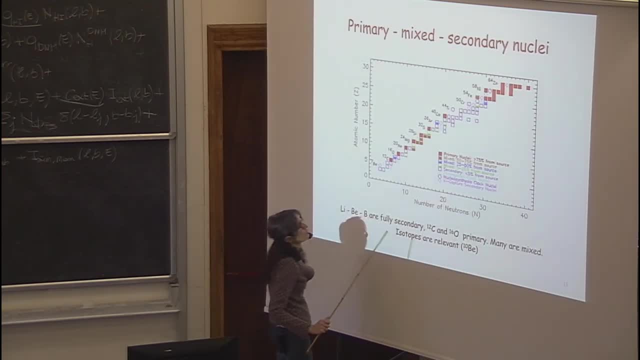 And this triangle here is propagation clock nuclei. Then there is the iron and very heavy nuclei. They are mostly primary And iron and nickel mostly can break on the interstellar medium and give birth to this number of isotopes which are called the sub-iron nuclei. 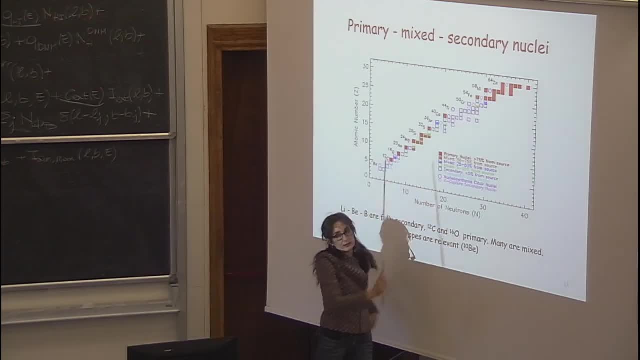 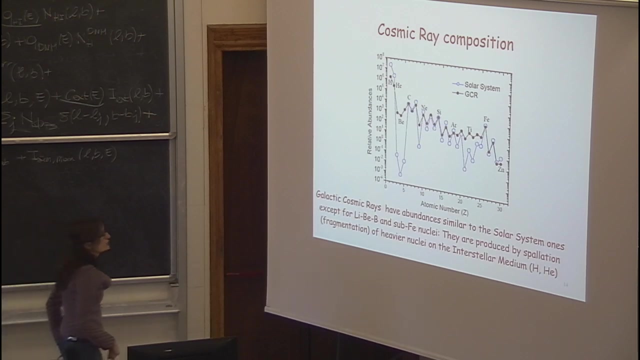 that are fully secondary. So this is a kind of screenshot for the parenthood of nuclei and isotopes in the Milky Way. Indeed, the fact that there are secondary nuclei in the galaxy can be also deduced in this way: These blue lines. 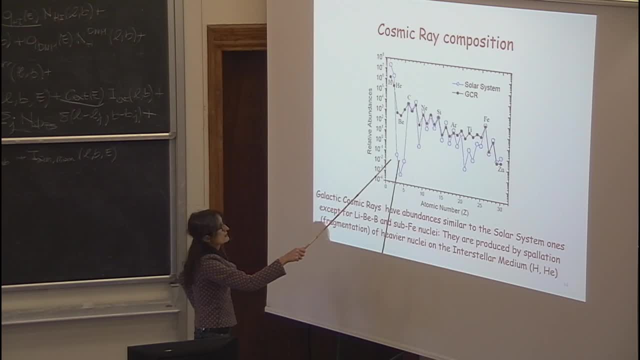 the blue line connects the abundances of the nuclei that you read here, so helium and hydrogen, lithium, beryllium, boron, CNO and so on and so forth. The blue line is for the solar system, from the solar environment. 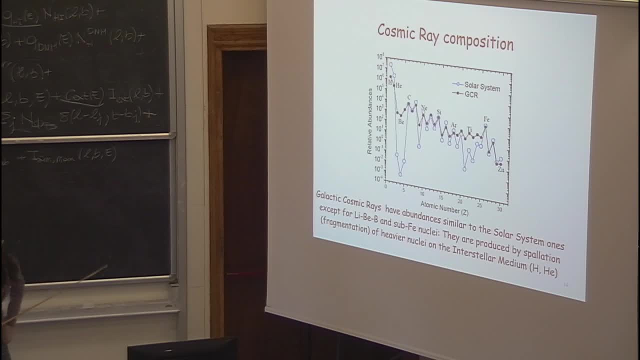 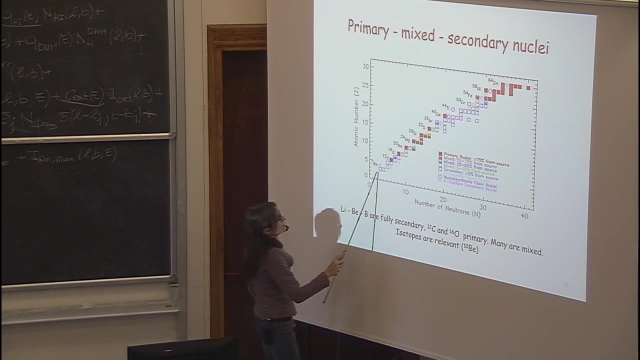 And in our neighborhood we don't have secondary nuclei. So the fact that indeed at the galactic level we measure secondary nuclei, in particular lithium, beryllium and boron- you can see here lithium, beryllium and boron- 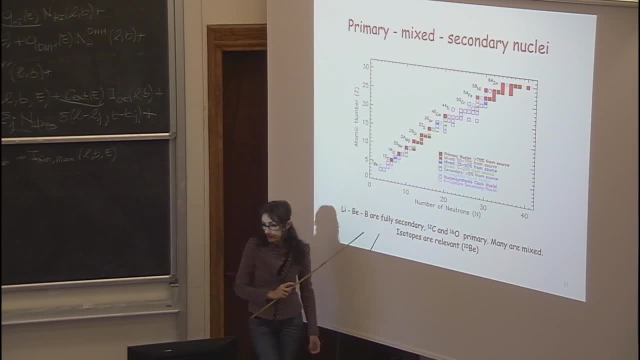 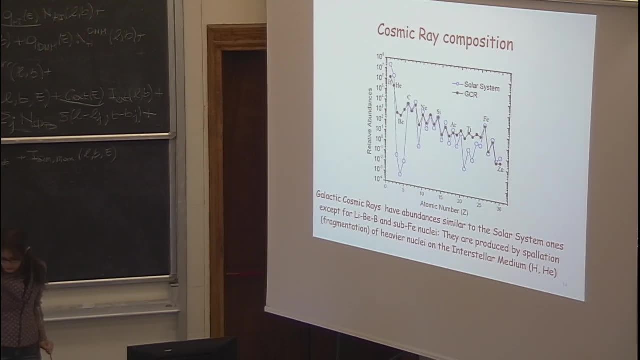 They are almost fully secondary. The fact that they are not present in the solar system for lithium, libeb and also for the sub-iron really means that there is a mechanism in the galaxy that permits the creation of these secondaries, and so far we understand it. 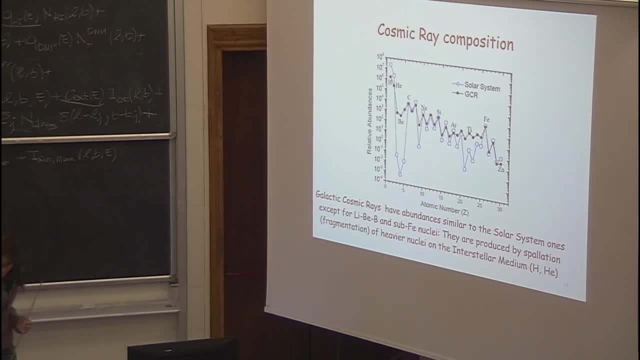 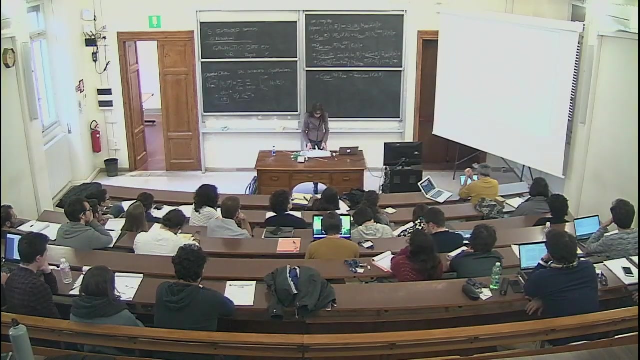 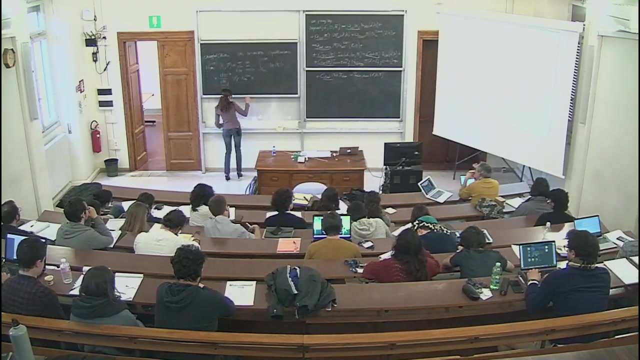 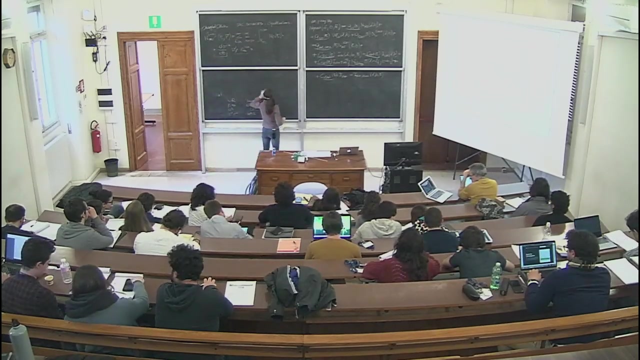 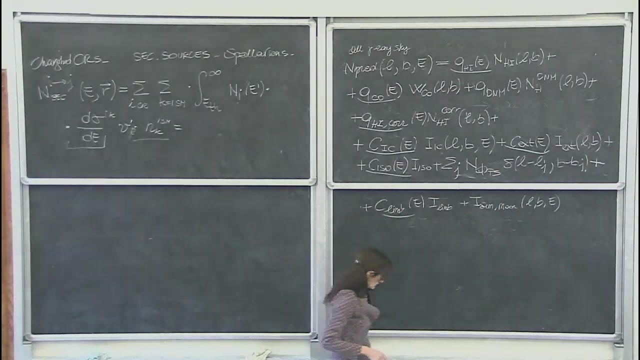 as spallations of heavier nuclei. Okay, So now I briefly go back to the transport equation that we have seen a few times and try to give you just some very indicative tools In order to solve it. So I don't write the transport equation once more. 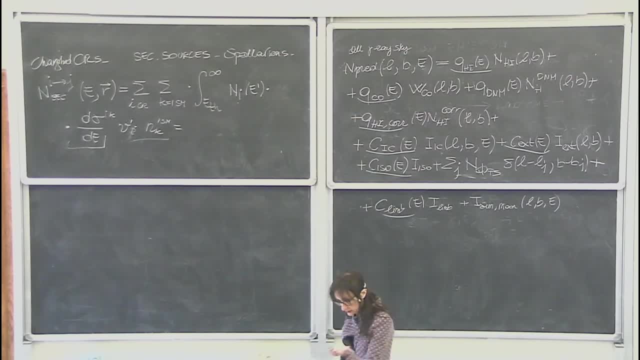 You always have it in mind or in your notes. It is an equation which is, in principle, is three-dimensional in space and there is a coupled equation in energy which is- I derived you a second order differential equation, also in energy. 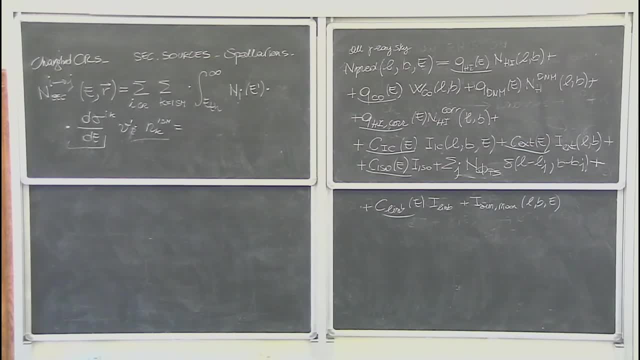 to keep into account re-acceleration and, at first order, also energy losses. So how can we solve it? Well, in principle you can do a numerical solution, So solving numerically both the space and the energy part. Anyway, 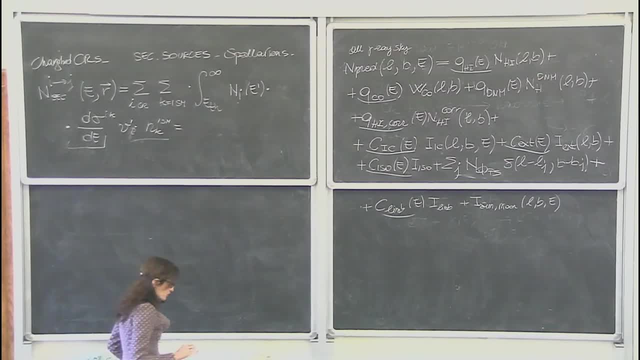 whatever is your solution scheme, you must make an hypothesis on the geometry of your galaxy, because you have to decide where to put re-acceleration, where to put the sources, where to put the interstellar medium. So a way of seeing our galaxy. 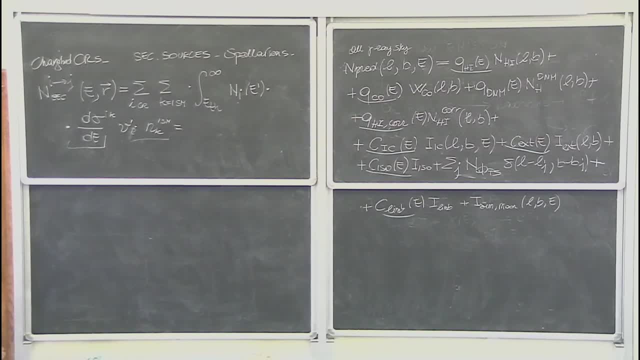 from a cosmic ray point of view is to imagine it as a cylinder. And well, of course, my picture is a bit. You force me to use the blackboard and then I have very bad pictures. I'm sorry, But it is very easy to put. 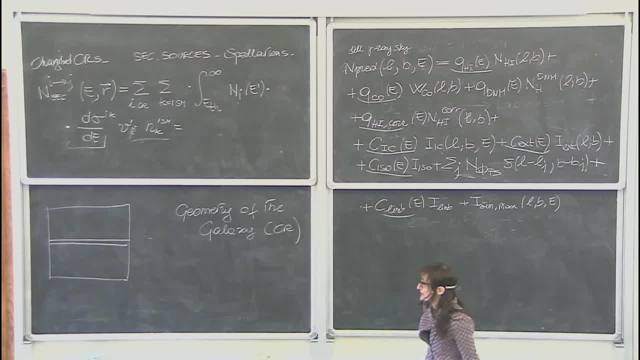 keywords on Google and to find better explanations. But we derived together so it is maybe easier to understand and to memorize it. So this is the galactic disk Where we have sources and gas, All the sources and all the gas that I described you before. 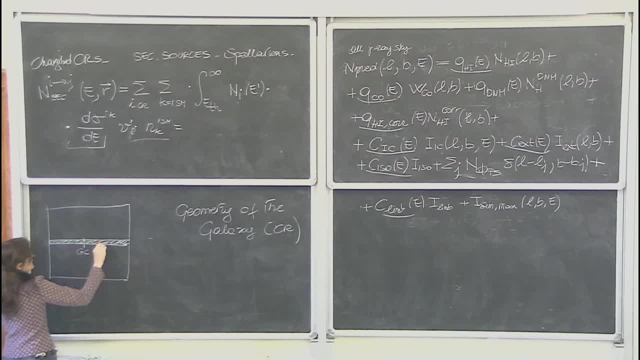 This is the galactic center. This is our position. The radius of our galactic disk is about 20 kilopassecs And the thickness which I call H- usually H is the half thickness- is 100 parsecs. So 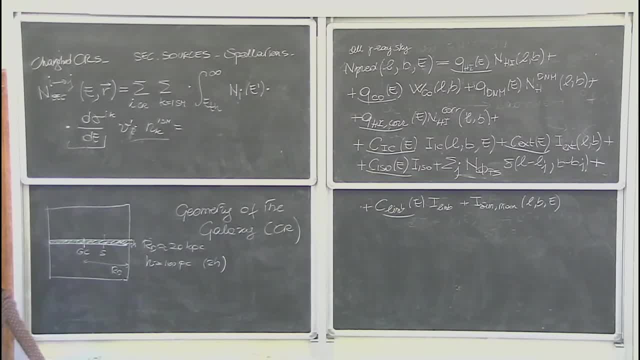 the full thickness is 2H. This is an approximation, but just to give you the numbers that are typical for this situation. And the distance of the Sun to the galactic center is about 8.5.. So this is the distance. 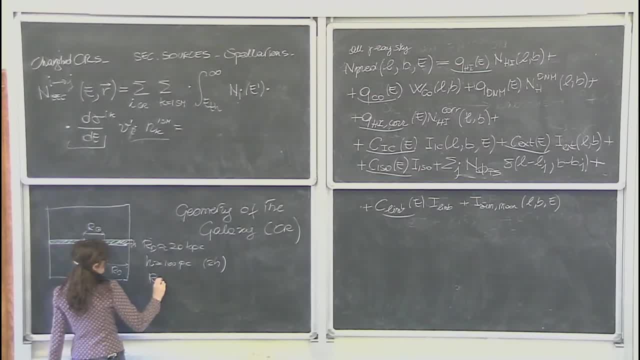 to the galactic center, And it is more or less 8.5 kiloparsecs, according to the years, of course. And then there is very likely, we are almost sure about that- we cannot avoid to include this zone of the galactic center. 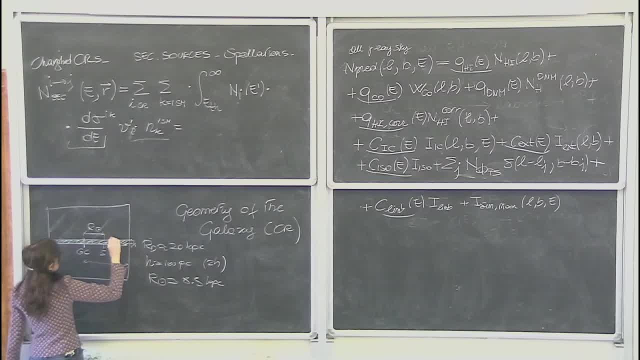 because this zone is above and below the galactic disk, in which the gas is very rare, but that is not true for the magnetic disk, for the magnetic fields. This is mostly evident for external galaxies. I was in this a few lectures ago. The fact that we measure 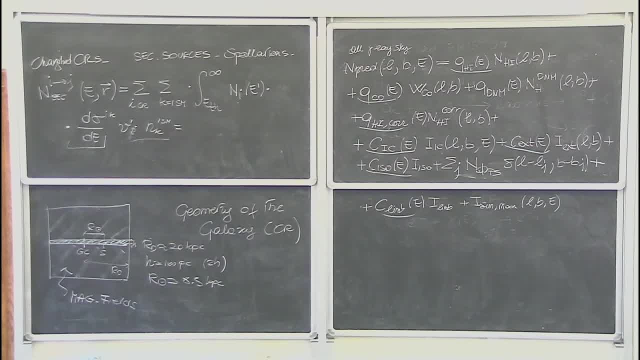 radio emission at high eighths from the galactic planes of some external galaxies. That means that if there is emission at radio wavelength there is some very likely synchrotron process taking on and then magnetic fields. If there are magnetic fields. 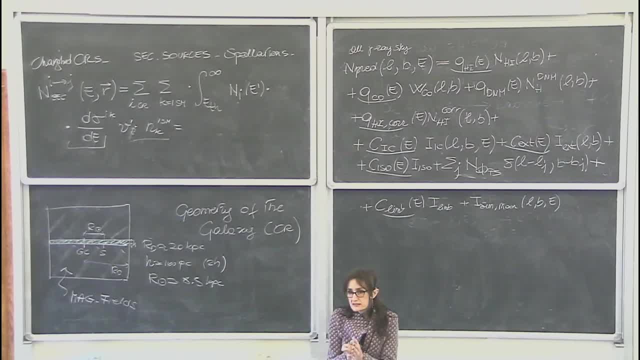 our particles run in these magnetic fields, So the diffusion coefficient and the transport of cosmic rays happens everywhere, Also in this diffusive zone which is called the halo of the galaxy. Then there are many halos because there is this diffusive halo. 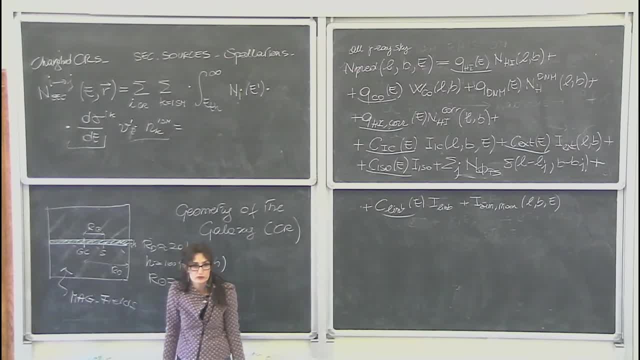 and there is also the dark halo, so don't confuse. And when solving the diffusion equation, one has to evaluate where all the processes occur. We have the disk and we have the diffusive halo. This is one way of modeling the galaxies. 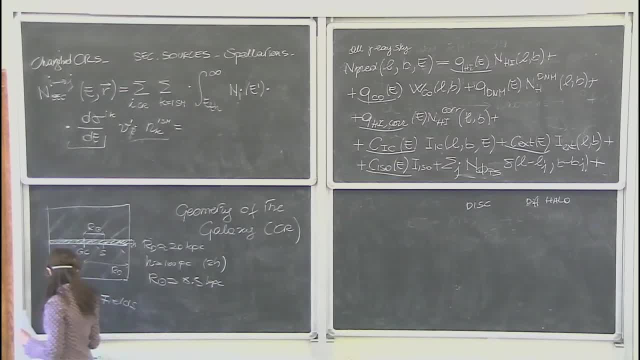 It is not the only one, but of course it is the simplest and, to the aim of our lectures, also the one that gives you the most easy understanding. This is used by several groups, indeed, when solving the transport equation. So 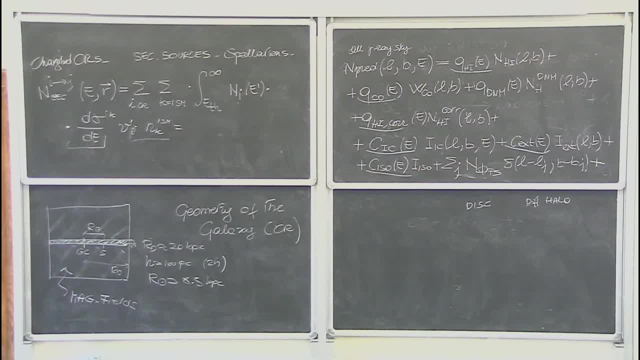 it's not only a toy model, it is a realistic model. So this is the diffusive halo and this is the disk. The eighth of the halo is not very much visible to the eye. So this is the diffusive halo. 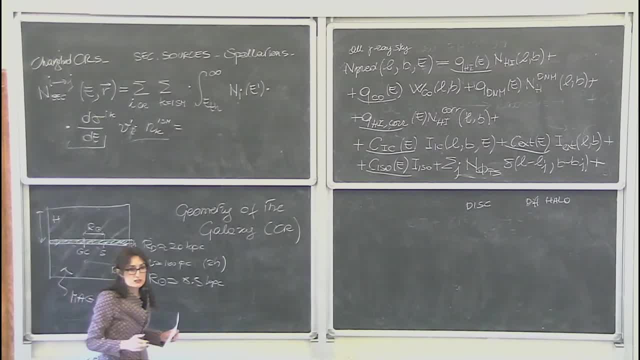 The sixth halo is not very well determined. Anyway, it is of the order of at least a few kiloparsecs, Let's say two, maybe five. even ten kiloparsecs is still. I think it is still possible. 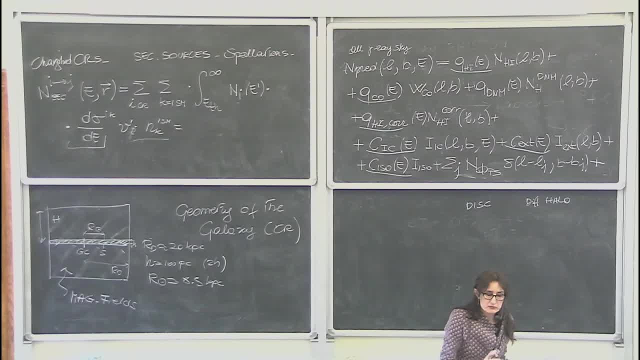 isn't it? Yeah, Indeed, we are. I mean recent analysis, favor high halos than very small halos. So it is probably to exclude one kiloparsec halo, but ten kiloparsecs is not very much visible. 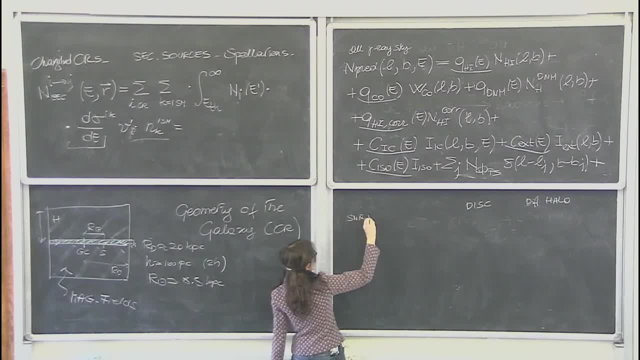 So, if you have in mind the diffusion equation, we have sources, primary sources In this scheme. they are in the disk and they are not in the halo, And then we have magnetic field. magnetic fields that mean diffusion, and diffusion is everywhere. 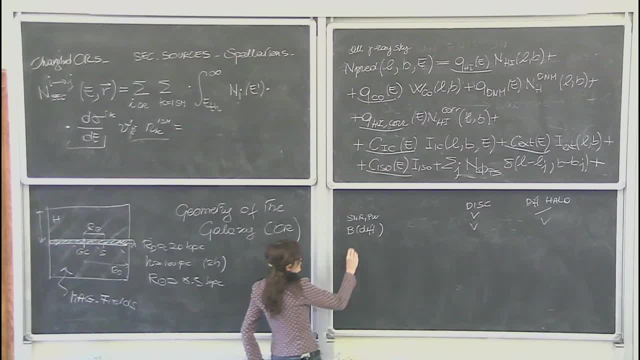 So it is very likely that there is a gradient of the convection velocity And then we have convection. I was maybe not very detailed on this. Anyway, you remember there is a gradient of the convection velocity. Anyway, very likely. not very likely. convection is everywhere in the disk And it can also be set in the halo. There are different ways of modeling reacceleration, But mostly, of course, it is in the disk where the magnetic turbulence is very high. 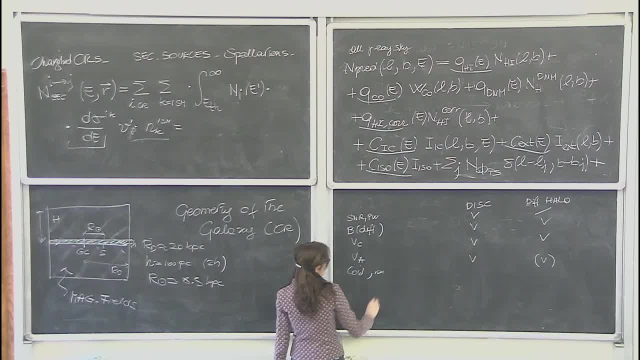 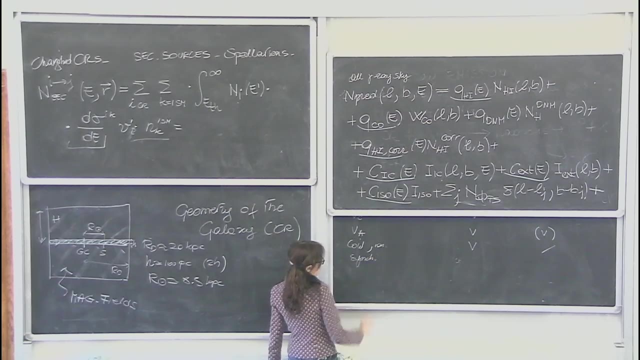 Then there are Coulomb and ionization energy losses. This is because there are no targets. Then there is synchrotron emission, let's say synchrotron energy losses. Since magnetic fields are everywhere, this must be set everywhere. And 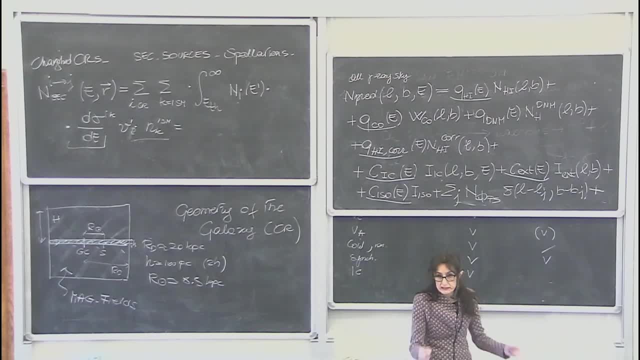 then there are other elements that propagate also in the diffusive halo, And at least the CMB is in the halo. These are, I'm discussing here the losses, And then if you want to make even bigger halo than the diffusive halo. So 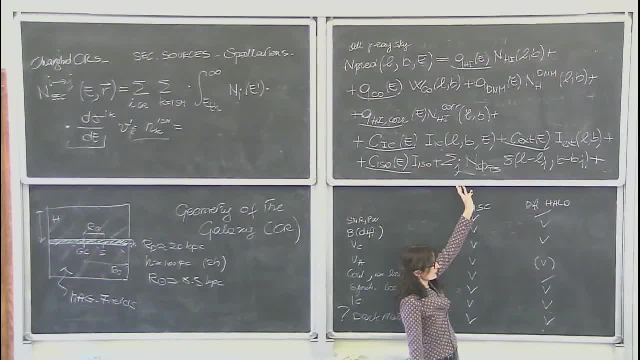 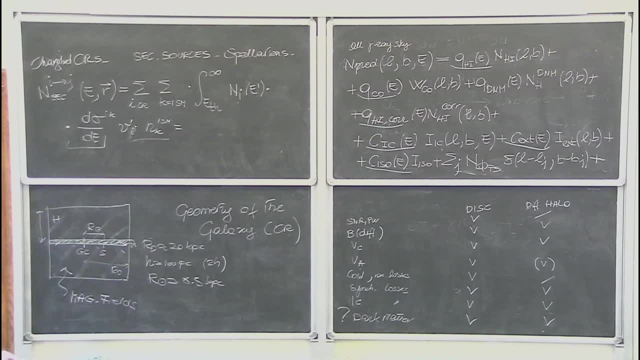 that's sure that that matter. if it is, there is everywhere. So when solving your transport equation, even if you have made the solution, because, for example, you see that energy losses some are only in the disk, some are everywhere, And the solution 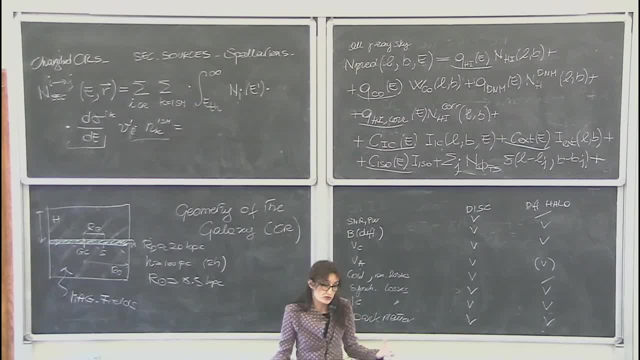 is not that easy. In fact there are few groups in the world that can solve this problem. So for one species it is a bit more easy. Anyway, given this cylindrical symmetry, there is one mathematical help. So if cylindrical symmetry is, 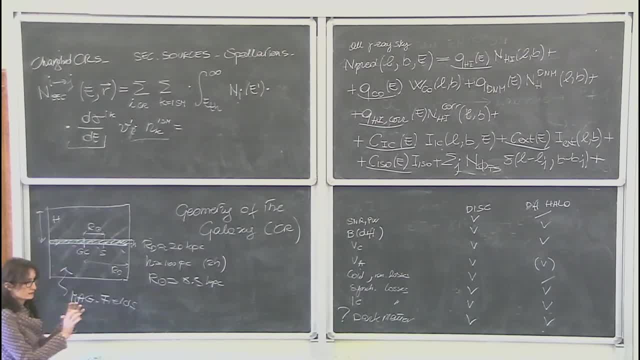 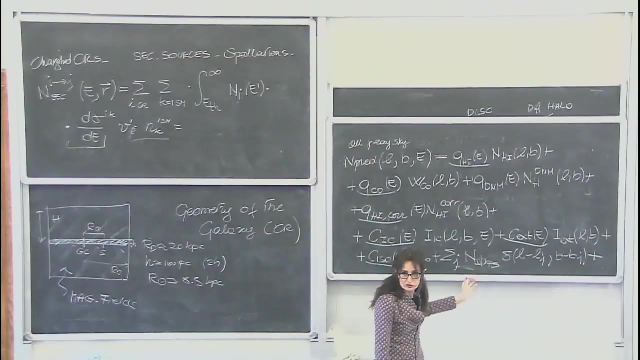 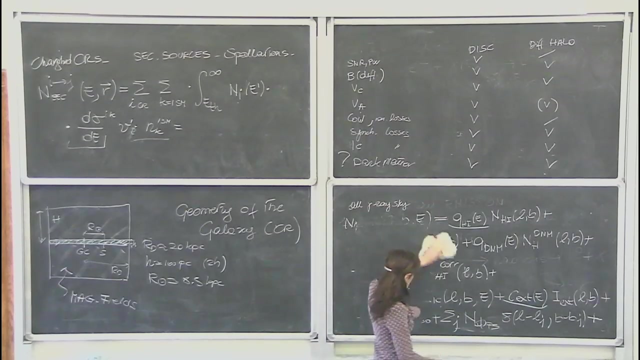 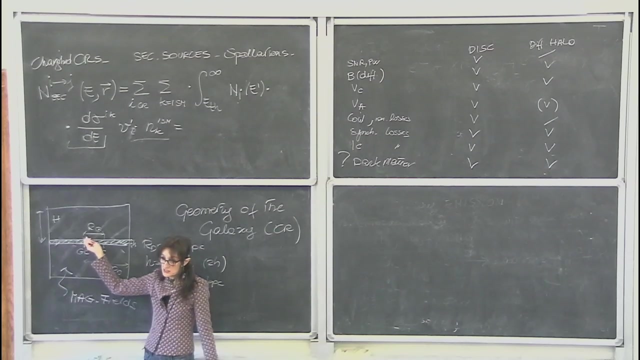 the same as the cylindrical symmetry, then it is much easier to solve this problem than to solve this problem. So that is the answer to this question. So, in this simplifying assumptions in which the gas does not depend on R and Z, and you. 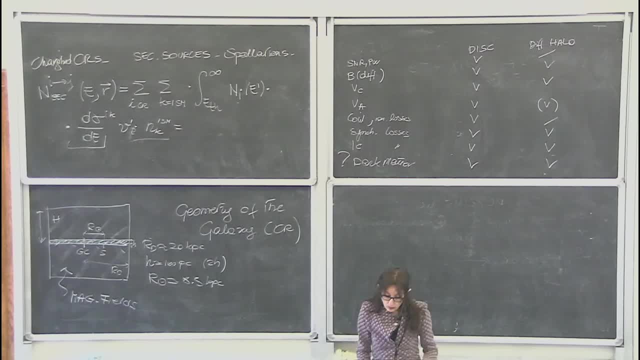 put a number. you say that hydrogen is almost one per centimeter cube and the basis in cylindrical symmetry. So in this case one can, first of all, for these simplifying assumptions I told you, imagine that there is a symmetry on the 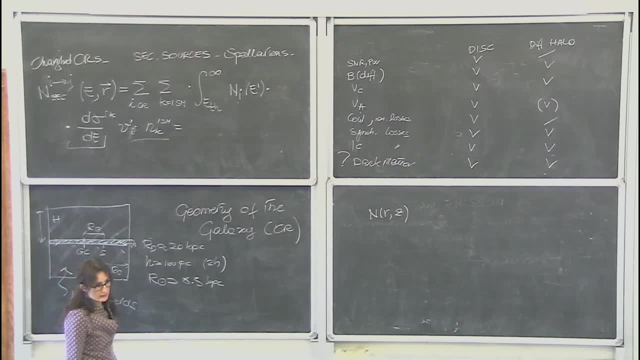 disk, And then the two coordinates that we are working on are R, which is the radius on the disk, and Z, which is the vertical coordinate And the function of R and Z as a development of a function which is a function of Z. 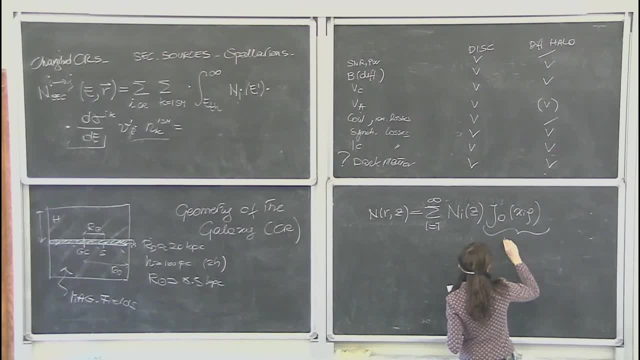 developed on the basis of Bessel functions And I have set rho equal to R divided by the maximum disk of the galaxy, which is this more or less 20 kilo parcels, And these J0 are the Bessel function of order zero. 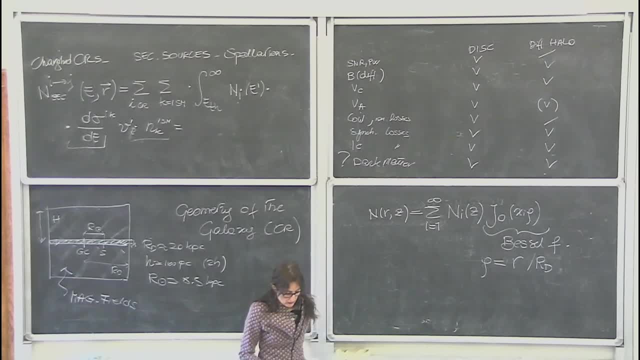 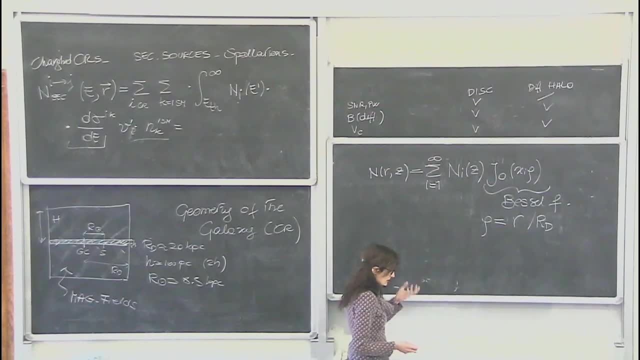 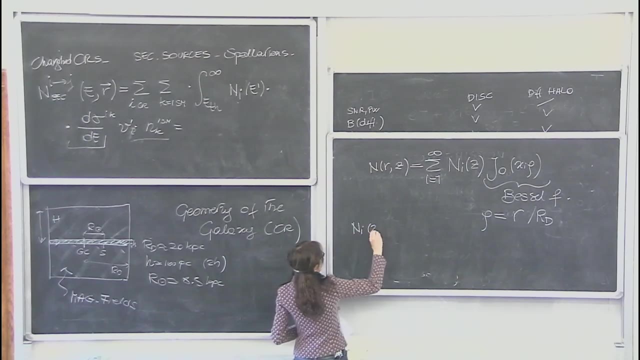 And Xi is equal to Z. So you can solve it analytically in this hypothesis and find an expression for an I of Z. And maybe it's not worth that, I think, if the sources are Q, disk, R and they are set to zero out. 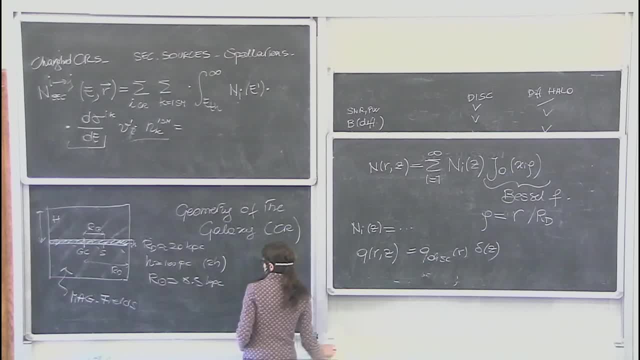 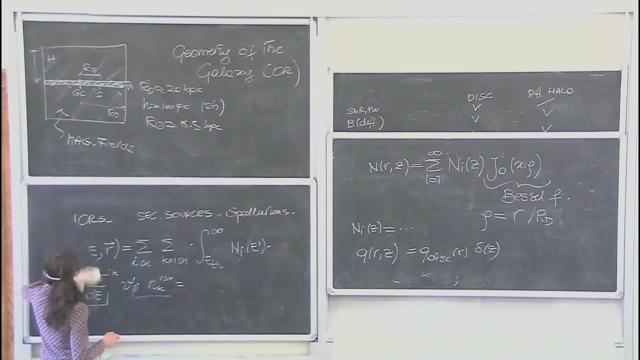 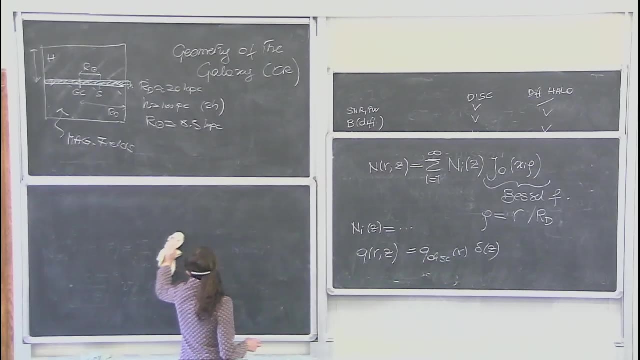 of the disk. This is true for supernova, remnants, pulsar and spellations in the atmosphere, So you can write the full solution you can derive by yourself. I want to write the full solution because it gives us some hints to the physics. 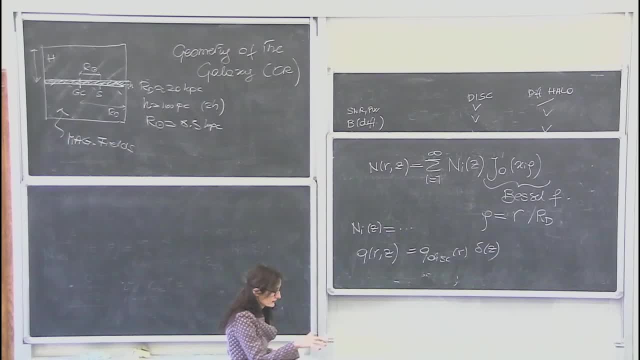 that we need to understand. On the other side, if you want to understand which are the main processes in this propagation history, it is easier to see than just a full numerical solution in the distribution of cosmic rays as a function of rz in cylindrical symmetry. 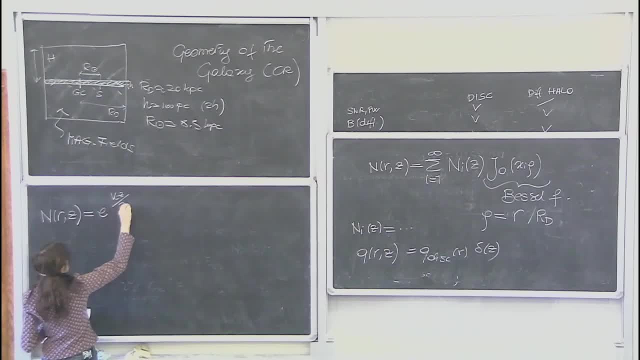 And the solution is this way: We have an exponential vc over 2k And then we have the hyperbolic sinus of a vector which is si l minus z divided by 2, normalized to the hyperbolic sinus of a vector which is: 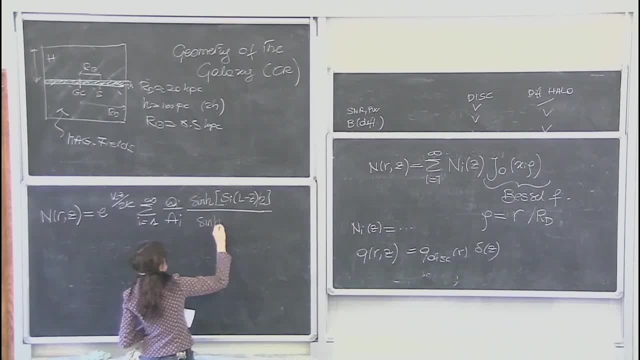 si, l minus z divided by two, And this is of course multiplied by j, zero, xi, rho. Now, this q is linked to the term source, so I don't specify it, but it is usually a normalization times, an energy dependence, And this factor that you 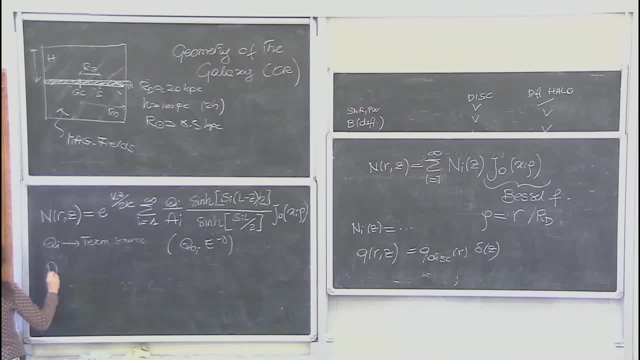 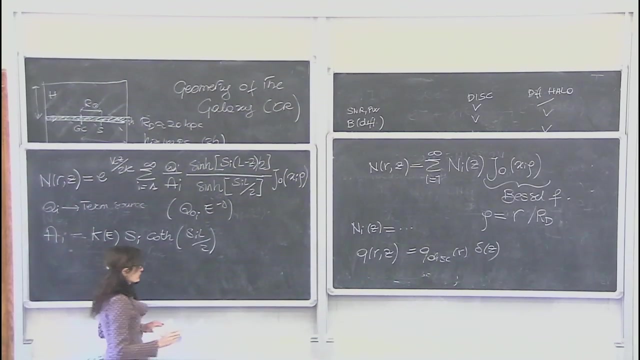 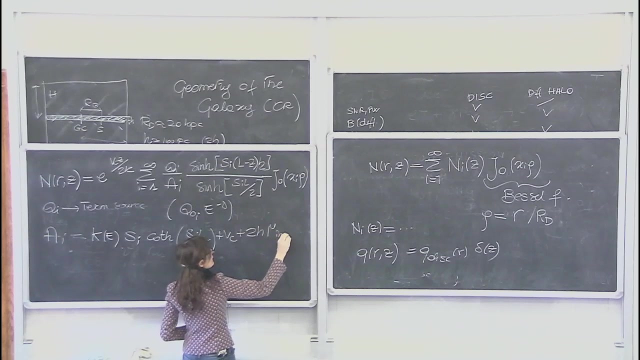 see here, ai is given by the diffusion coefficient. now I put the energy dependence by a term which is i hyperbolic cotangent s e l divided by two. And then there is another contribution, which is convection and the presence of inelastic destruction. 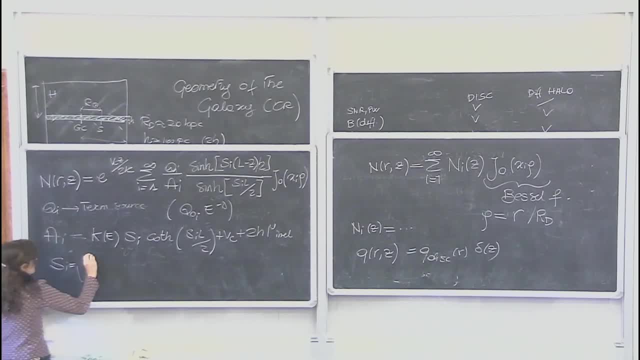 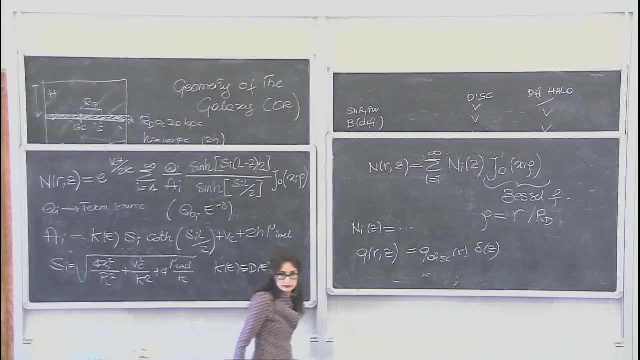 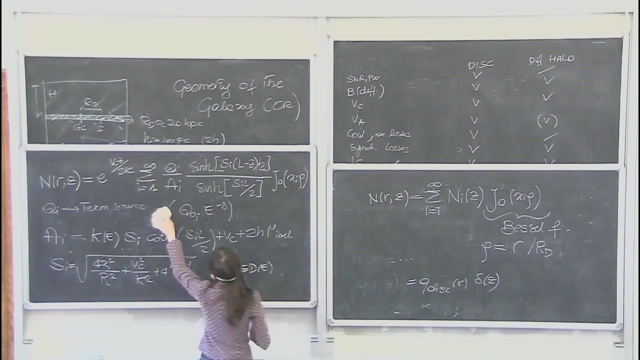 And this s e comes out to be four times the zeroth of the best function squared divided by r? squared plus convection squared, diffusion coefficient squared. and then there is a term which is our diffusion coefficient. I can maybe elaborate just a little bit on this. 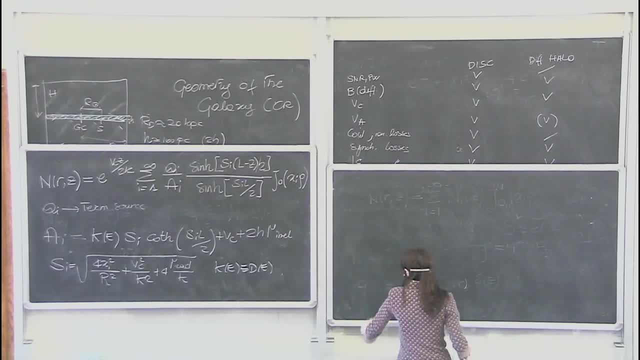 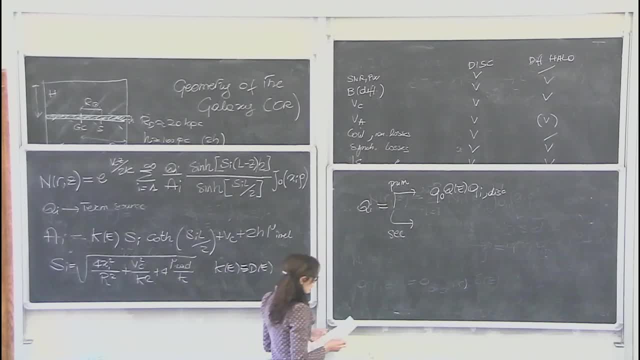 the development on vessel basis. So I mean a secondary one. Now I just change a bit the letters, otherwise there is a confusion. but anyway it is all the nuclei that give you this specific nucleus by spallation. So q e disk is the nucleus. 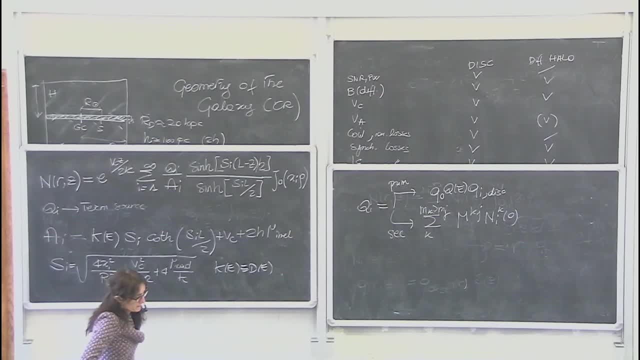 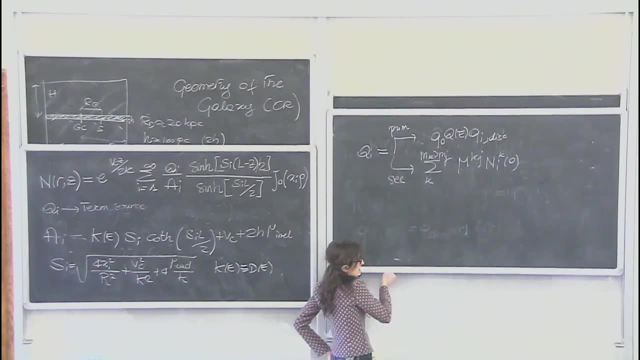 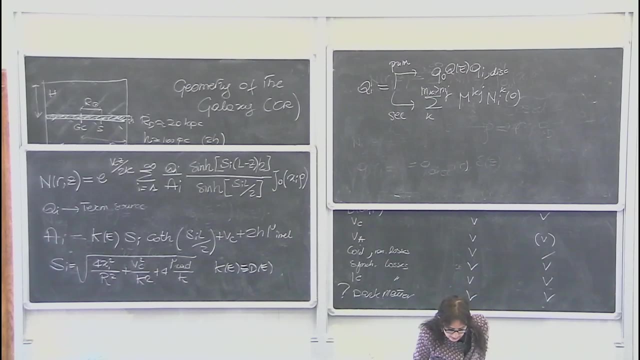 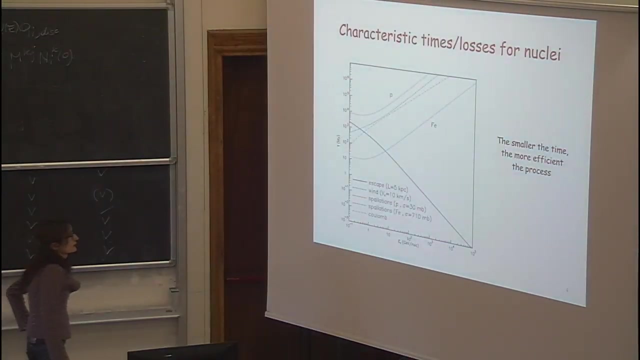 So you may be remember, I can probably also go back to this situation that we have seen together, The situation here. this figure tells us that we have a very short time for protons. Diffusion dominates, okay, which is this time, which is very short. 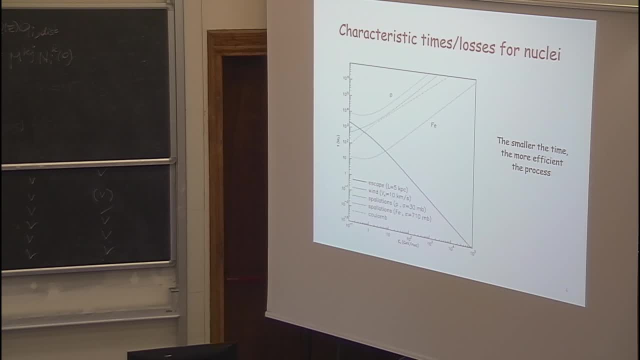 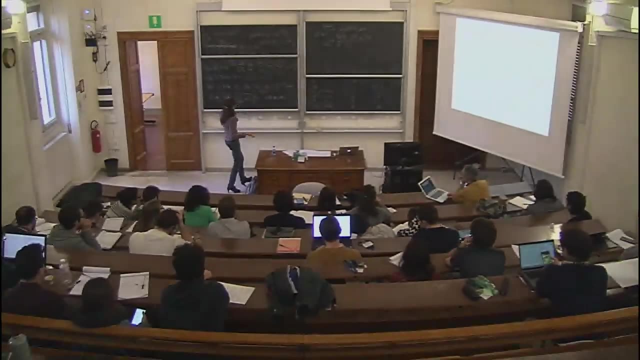 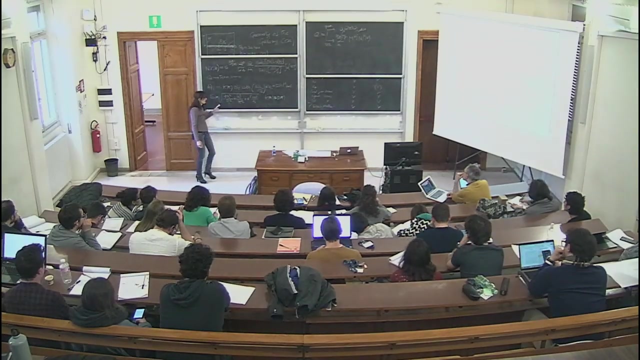 For iron, it is true, but only for higher energies. So the number of these terms can be put to zero. For example, this SI here. if convection make this hypothesis that it is not very relevant over diffusion, This goes to the physical processes. It. 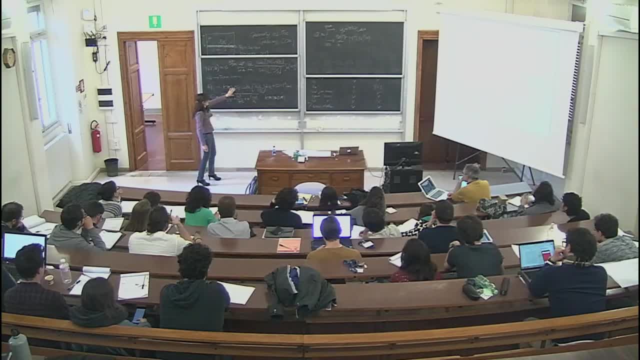 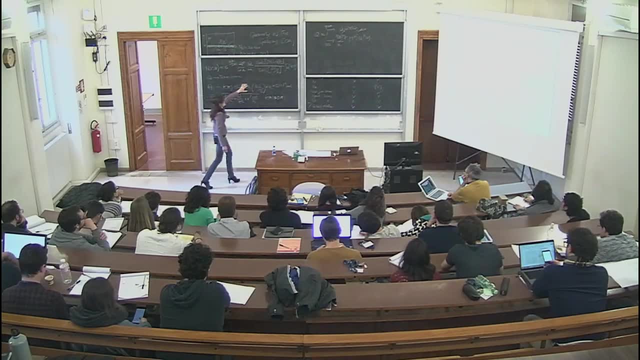 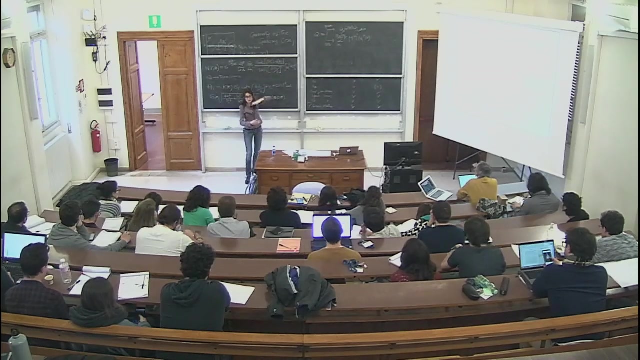 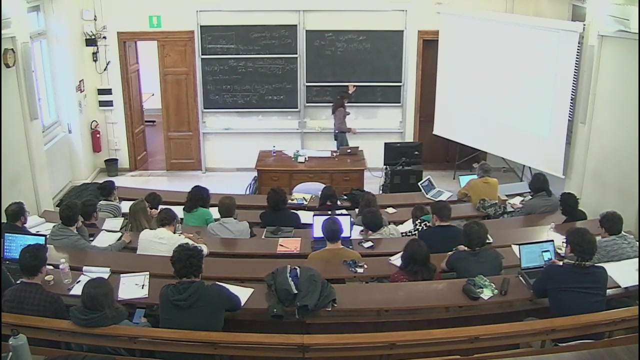 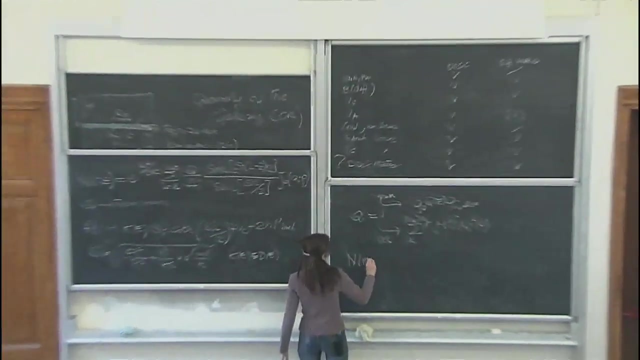 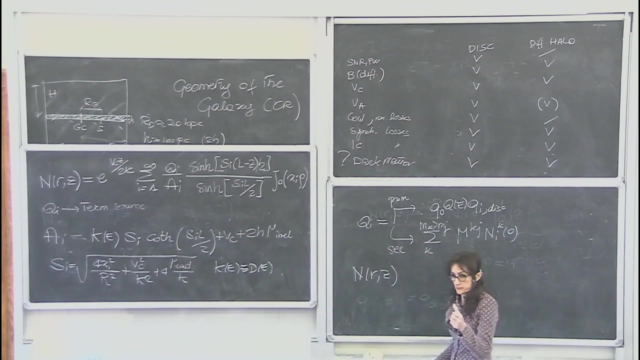 doesn't bring any special information on the physical processes. So in this case SI is a fixed number And so this is a number, and also this term of L is high. But in a very approximate case in which diffusion dominates and the nucleus is a, 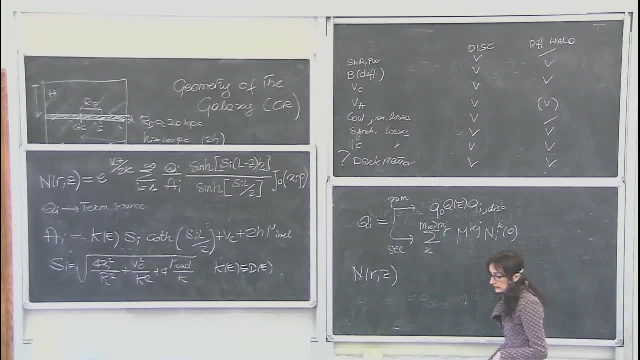 primary one, a proton, a helium, a carbon. then this quantity goes more or less as let's say it is. maybe it's better to write that with A, I, Bessel function. And this is proportional to Q of energy and inversely proportional to the diffusion coefficient. 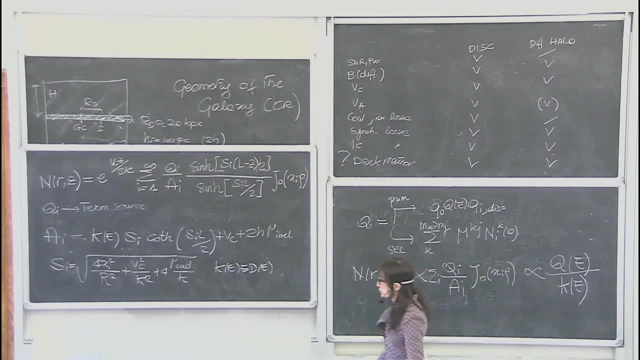 This was what I wanted to do. This quantity here is not energy dependent and it is mostly linked to geometry. But you have this Q, which is the source, and this A, which is, if this is negligible, and less factors, of course, But this gives us. 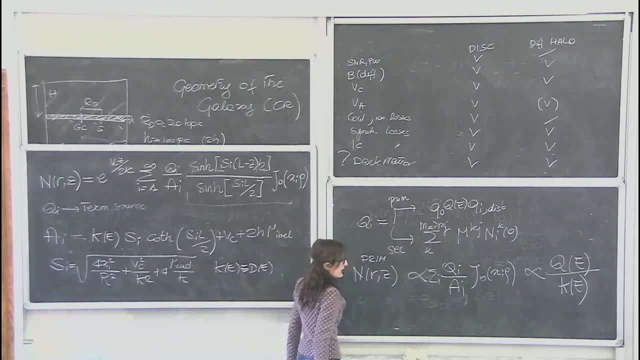 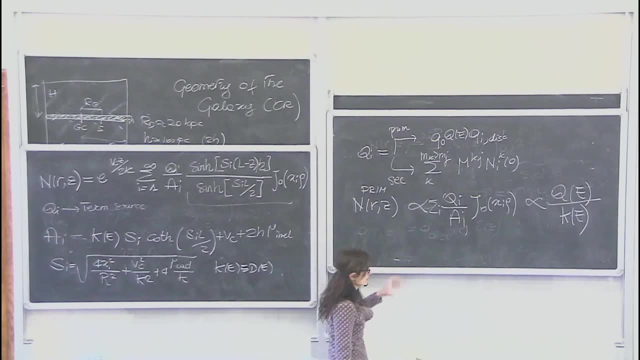 the trend of primary nuclei as a function of the energy. This is a very important physical insight. If the source is a supernova with the first order Fermi acceleration, this quantity here goes as an energy minus gamma Gamma. we don't know exactly. 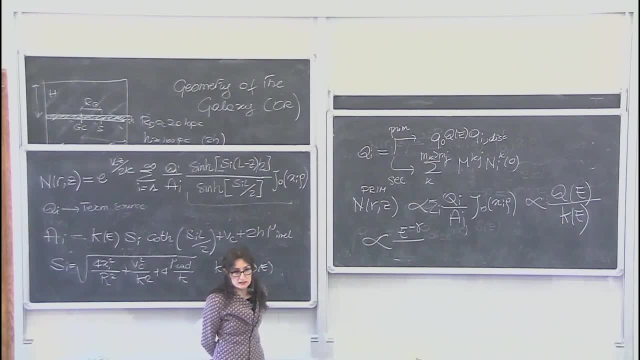 I told you that it is probably close to at high energy. it is the rigidity to delta. we defined it And so it is E to delta. So we expect that in the first approximation primary nuclei follow a power so measuring a proton at high energies. 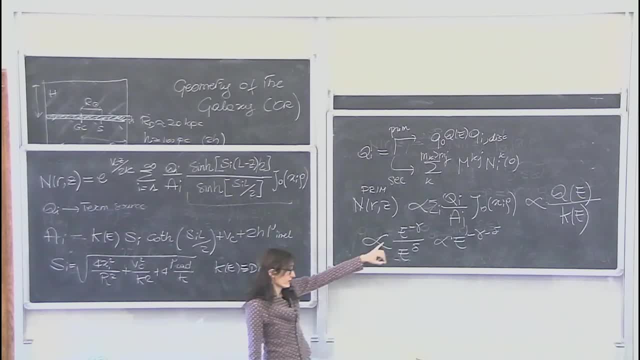 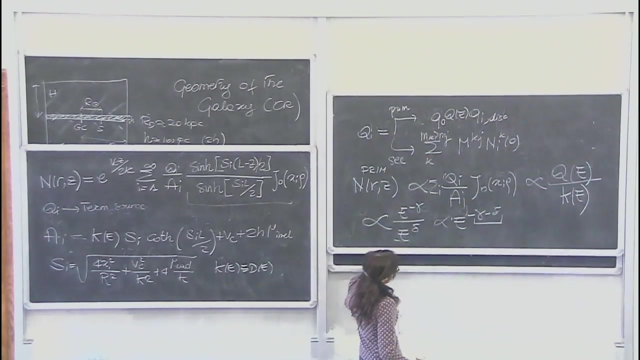 is first of all informative on its energy at source, the injection spectrum at source and the diffusion in the galaxy. But if we look at the energy of the primary nuclei, we can see that the energy of the primary nuclei is equal to the energy of the primary. 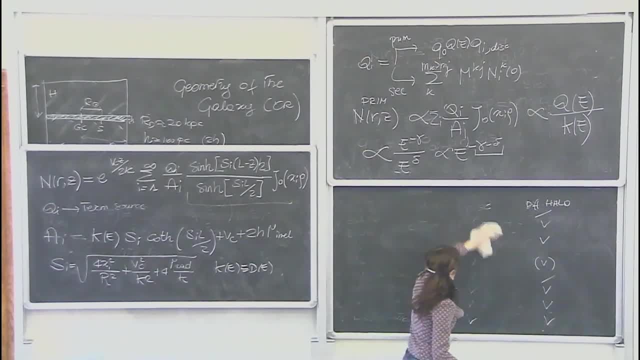 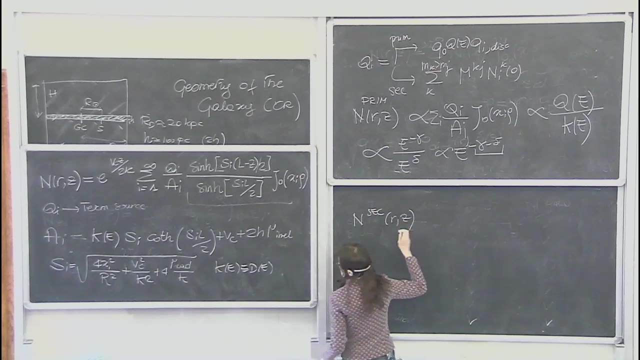 nuclei at the second nucleus Instead. let's keep this approximate reasoning. If instead we try to study a secondary nucleus, neglecting all the small or any other effects in the galaxy, this Q is a secondary source And the secondary source written in a let's 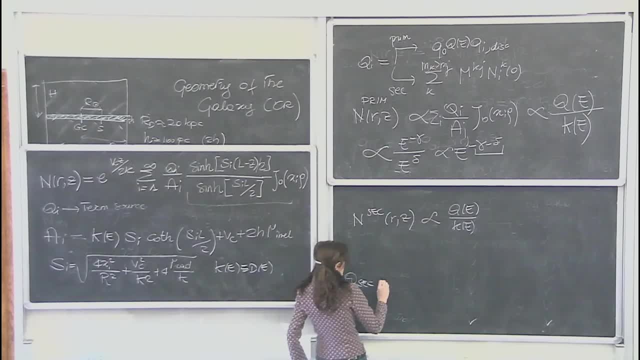 say a bit quick way- is proportional to a cross section which produces this nucleus, The interstellar medium. but the energy dependence is mostly. there is some little dependence on the cross section but at high energy it can be neglected. It is dependent on the energy of. 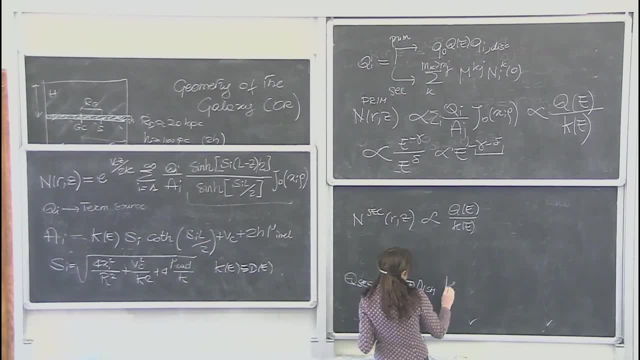 the nucleus. But then there is the spectrum of the parent nucleus And, again at a good approximation, the parent is the primary. It's a carbon, it's an oxygen. So let's write: this is the diffusion effect on the secondary nucleus when it is. 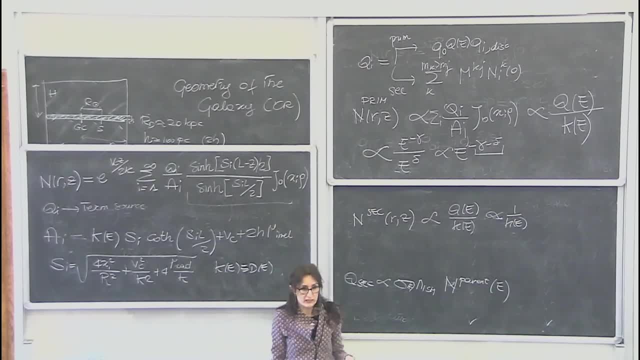 produced and starts going around in the galaxy, But its source is this one And this is this one. So more or less it is e minus gamma minus delta, e divided plus delta. Let me still write this way. So again, if you study this, 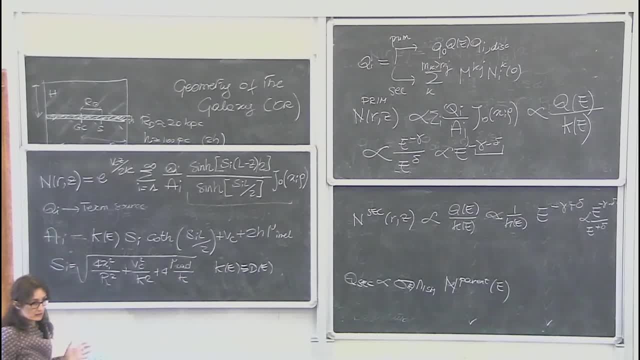 it's very difficult to disentangle diffusion properties from the rest of the processes that are affecting it, But a way to disentangle diffusion is to use the ratio of secondary and this one, Because the primary, more or less of course, cancel out. 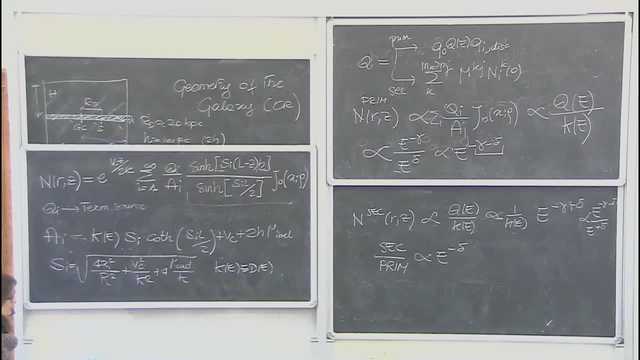 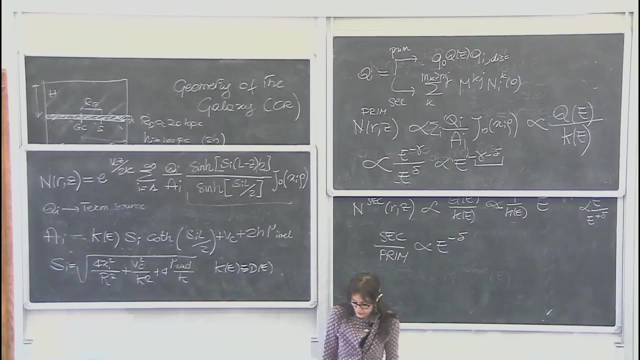 So this is a bit a rough way, but it can be some context, not a long time, as used. to understand diffusion, or to try to have hints on diffusion, is a specific ratio, which is the ratio of boron nucleus to carbon, The so-called B over. 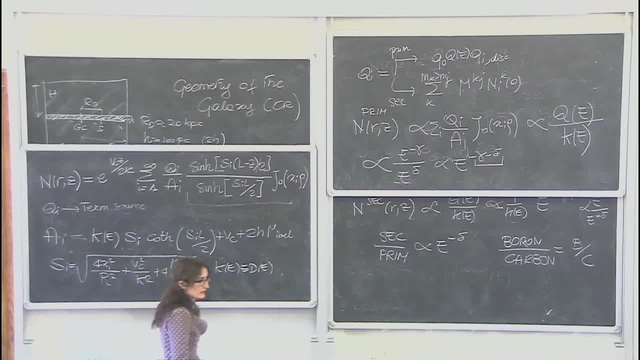 C. So this is more or less independently, and then published data on B over C. B over C has often been considered kind of standard candle for cosmic rays. So the quantity to which people who have these galaxies can be disentangled with B over. 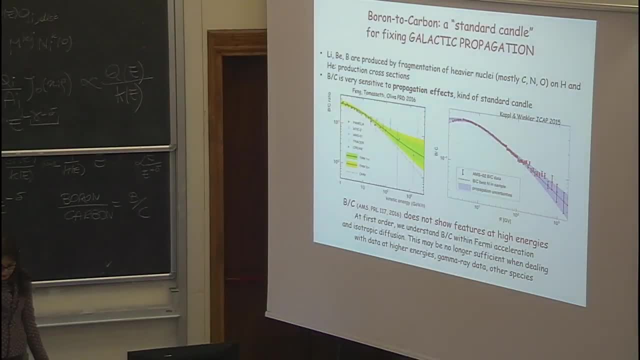 C And this is- you can maybe look at the right hand side- Many groups, including also the work I did in specific contributors. but what I want to show you is first of all this: at your right is the B over C measured by AMS. just very. 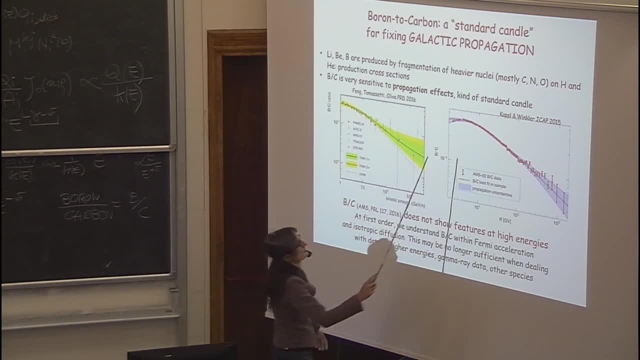 recently, very few years ago. So what you see is a very, very good precision. So also cosmic ray physics now is a precision physics. We have data till at least 1000 gigavolt in rigidity, and this is the first order we can. 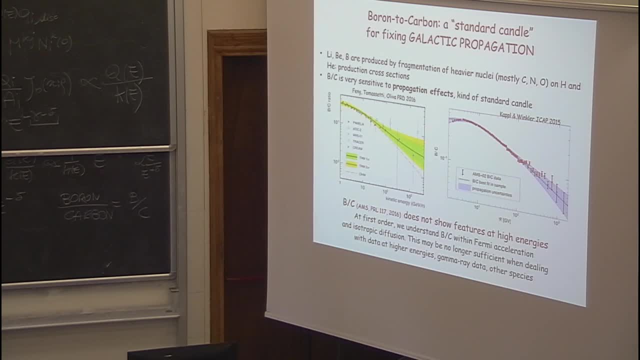 understand B over C using fermi acceleration and isotropic diffusion. Anyway, many data are arriving from space which do not only include B over C, but we have to refine a bit our models to interpret them. But this will be left, probably, to your research activity. 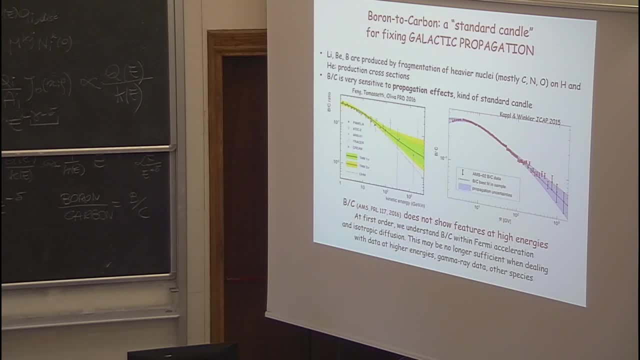 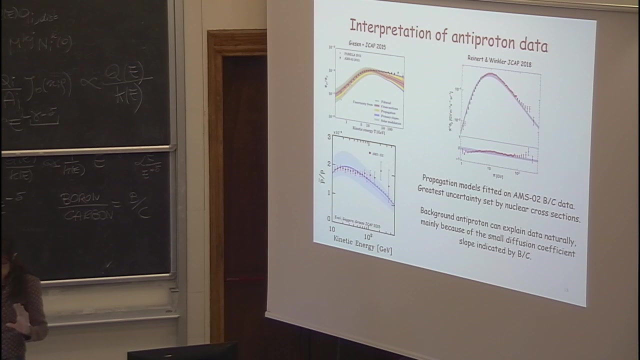 in your next years if you are dealing with it. So this is a very complex model and it is very complex, but then you arrive at the prediction and then you have data and this is a lot of fun. I just take one more minute and then. 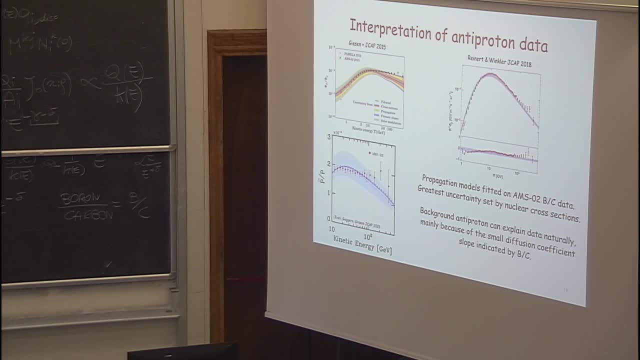 we close this lecture and we close the school. Among the secondaries, we don't only have the nuclei that I listed before. We have positrons, maybe anti-deuterons, even if we don't have data, and these are the secondary nuclei or anti-nuclear. 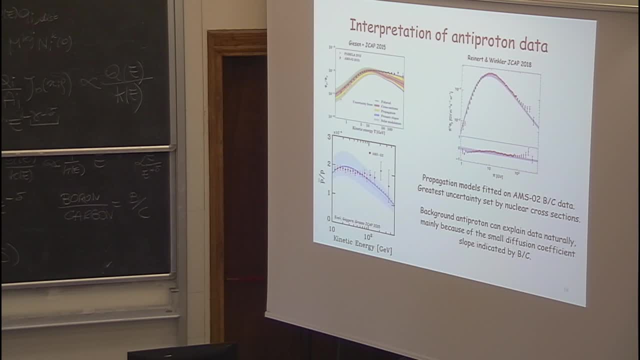 channels in which we also search from some dark matter modeling, And what you see here is some data. maybe better to concentrate on this, but the anti-matter channel is pretty interesting to see. the data are precise, So this also for you who are. 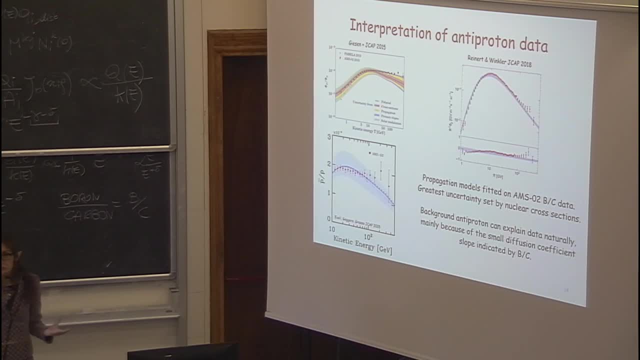 starting your activity in research- a lot of perspectives and surely a lot of fun. I just wanted to thank you for your attention and a presto In two minutes, because then I am going to go to the end of the presentation. Thank you very.